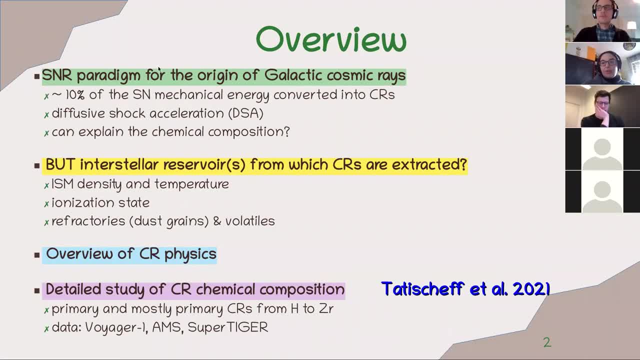 And in particular in our work we address the issue from which interstellar medium phase cosmic rays are more likely to get extracted by sources. In this talk I will provide first a brief overview on what is the so-called supernova remnant paradigm for the origin of galactic cosmic rays. 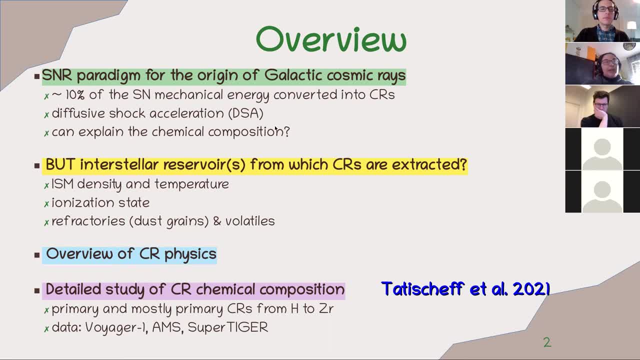 Indeed, in the last decades, there have been more and more establishing consensus on the fact that supernova remnants are likely the main sources of the bulk of galactic cosmic rays, which would be excellent for the creation of cosmic rays. And, of course, this is not all. 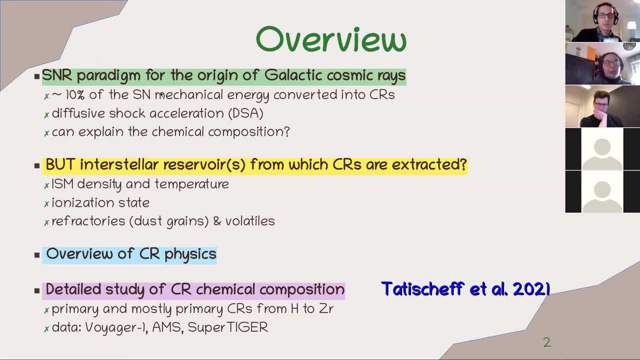 In the past we have accelerated that shocks through diffusive shock acceleration. This scenario is appealing for several reasons. First of all, from the energetic point of view, because it requires just an acceleration efficiency of 10% in order to explain the bulk of cosmic rays. 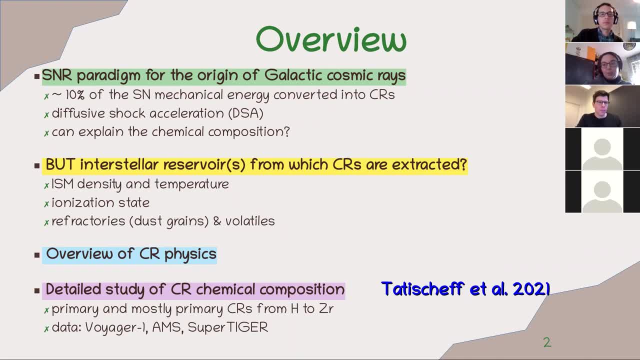 Moreover, diffusive shock acceleration, as we will see naturally, would produce powerless spectra, which is what we detect roughly, And also several details of the cosmic ray composition can be explained through supernova remnants. However, there are several issues that should be clarified. 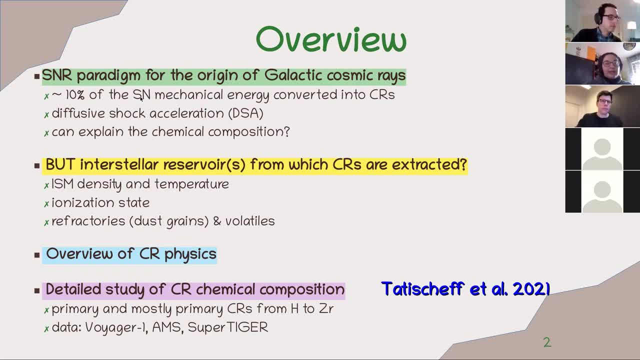 One of them is whether acceleration can proceed to very high energies. So this is one of the main issues of this hypothesis, but I will not address it. And there are another aspect which is mostly related to the chemical composition. Indeed, when we go through to the details of acceleration, it is still not clear whether the composition at the sources is well explained by supernova remnants themselves. 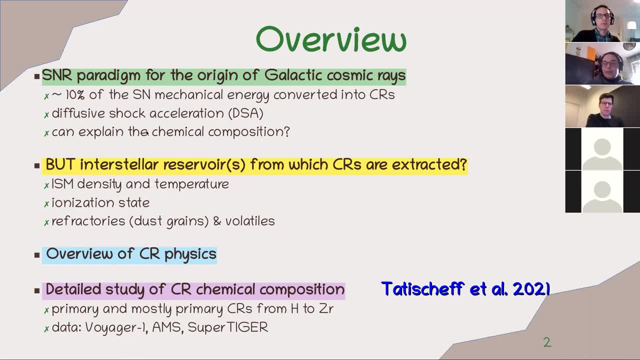 But also, it is not clear where supernova remnants accelerate cosmic rays, namely from which gas receiver they accelerate them, Indeed, they accelerate Indeed. the acceleration will depend on the ISM density and temperature, which provides, basically the ionization state of the particles that enter the shock to be accelerated. 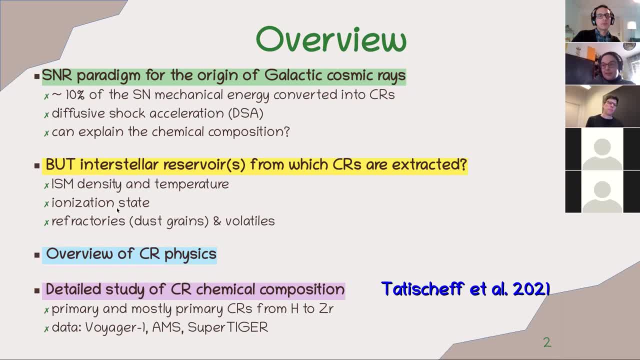 And so, depending on this ISM phase, the acceleration will proceed in a different way And, in particular, we will see that there is a very important distinction between particles that are in the ionization state and particles that are in the shock state. 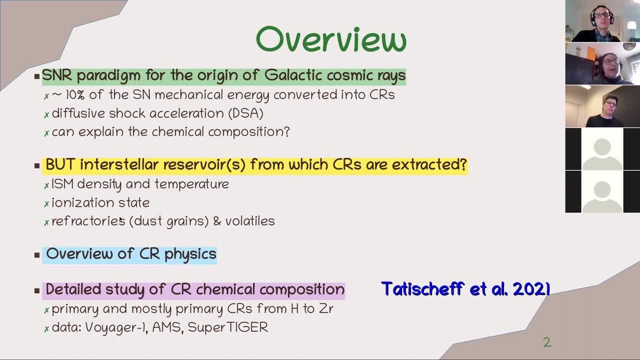 And so, depending on this ISM phase, the acceleration will proceed in a different way. Hence, we have particles that are in the gas phase and particles that are locked in dust grains, and for them the acceleration proceeds at a different efficiency. And so what we did with Tatischeff and others, 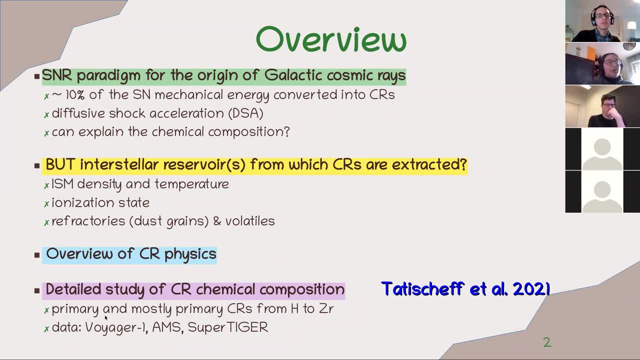 was to investigate the origin of primary and mostly primary cosmic rays, from hydrogen up to much heavier nuclei, using kamptu, using the Voyager-1 data, EMS and SuperTIGER, And from such data we extracted the very important information on the fact that probably 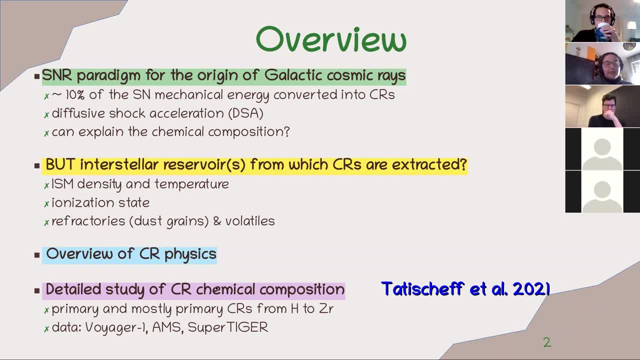 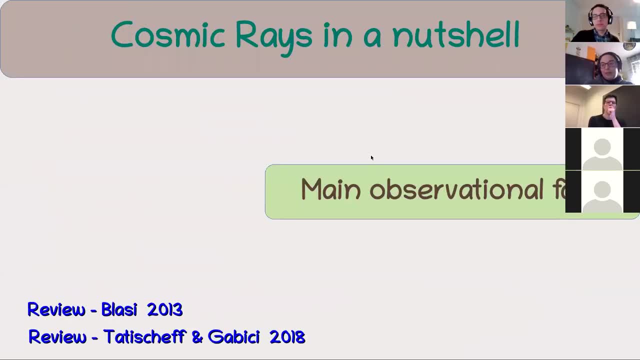 cosmic rays are accelerated from a super bubble environment, And this can be understood by looking at the composition. But now let's start with a brief overview on what we know about the origin of cosmic rays. For the readers that are interested in more details, I would suggest to look at the very 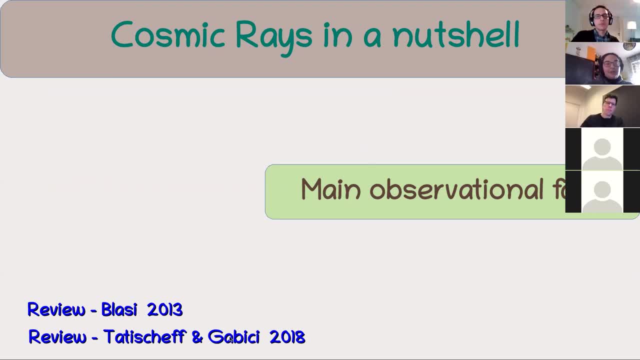 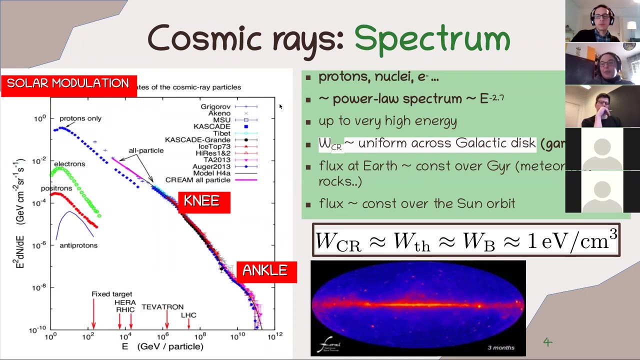 nice reviews from Blasi and from Tatishev and Gabishi. In particular, this review of Tatishev and Gabishi contains nice information on the composition, which is the main topic of the talk. So obviously, the first thing that we know about cosmic rays is their spectrum at Earth. 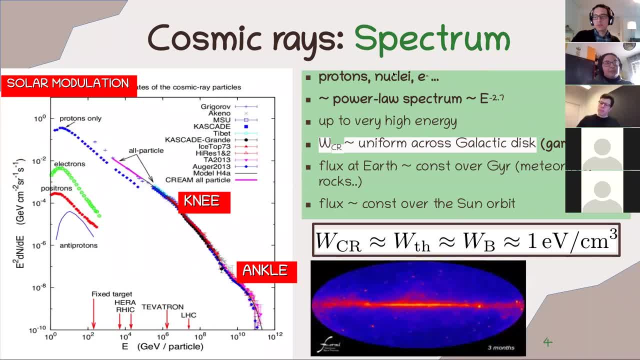 because we detect it And we see that most of these rays are in the solar system And we see that most of these rays are in the solar system, And we see that most of these rays are in the solar system And we see that most of these particles are protons. 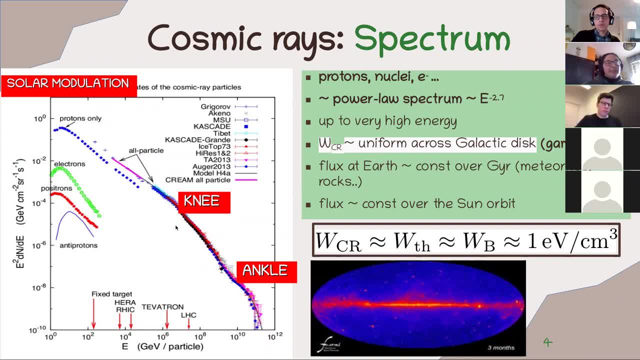 And cosmic rays exhibit a nearly power-low spectrum, with an energy spectrum of 2.7 s slope, basically extending for many energy decades. with some exceptions, In particular at PV energies, we have the knee where there is a steepening of the spectrum. 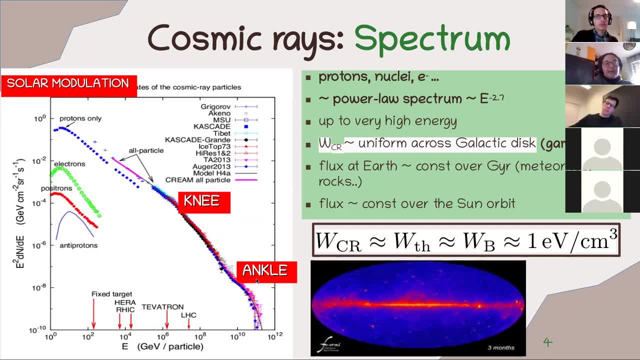 In particular at PV energies. we have the knee where there is a steepening of the spectrum, In particular at PV energies. we have the knee where there is a steepening of the spectrum. Another break: the ankle, is present at very high energies. 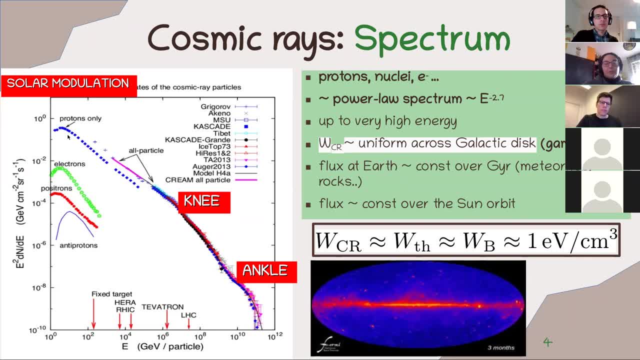 And then there is this part at low energies which is more difficult to understand because it's much affected by solar modulation, And so, in order to get a better idea of the low energy part of the spectrum, we had to wait until Voyager 1 exited the solar deliosphere. 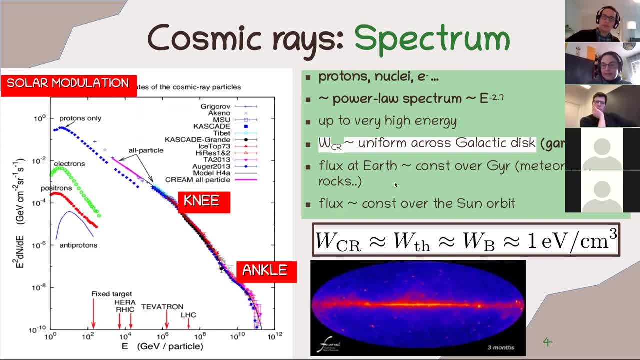 And then in the second part of the spectrum we have the solar deliosphere and so started to detect what is the local interstellar spectrum. In our analysis of the composition, what is really important is the low energy part of the spectrum. 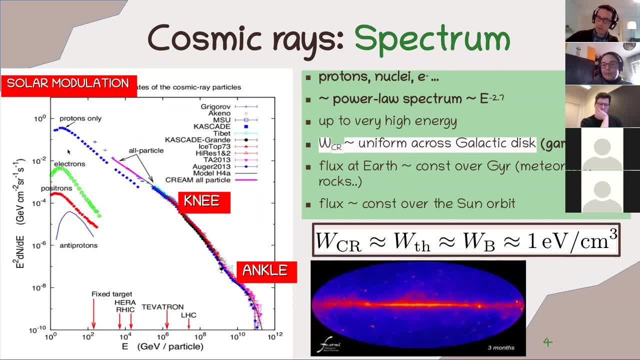 because we are dealing with a relatively steep spectra, also at the sources, And so the information on the composition, namely on the number of particles for a given species. it's hidden in the low energy part, which is the part that is not so well known. 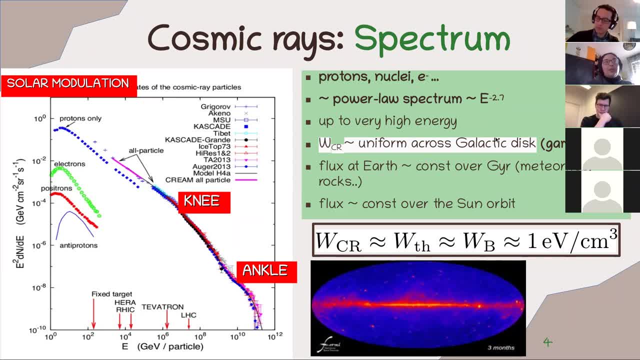 Then we had another very important piece of information, which is how uniform is the cosmic ray distribution across the galactic disk, And we get this information from gamma rays. Indeed, cosmic ray protons interacting with the ISM gas will produce neutral pions. 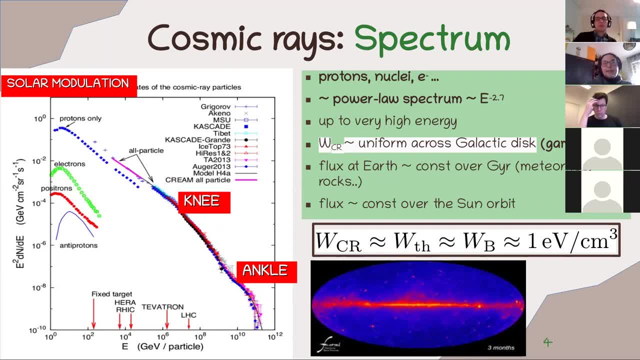 which decay in gamma rays. We detect such gamma rays as can be seen from this picture here, And from this information we know that the cosmic ray distribution across the disk is overall uniform, Plus from other information related to biological samples, rocks and meteorites, etc. 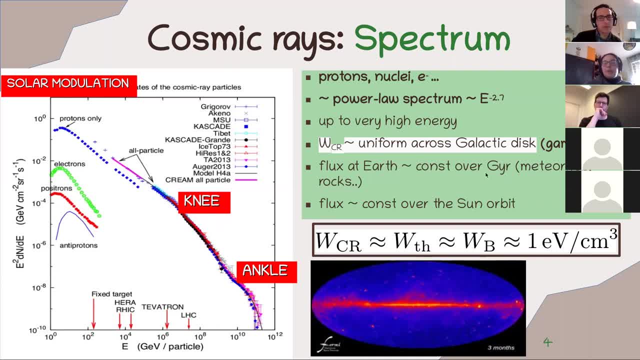 we know that the cosmic ray flux at Earth had remained constant over the last gigahertz and so also a lot more. So we can see that the cosmic ray is also in the orbit of the Sun in the galaxy. Finally, the cosmic ray energy density is overall in a quick partition with the thermal energy density. 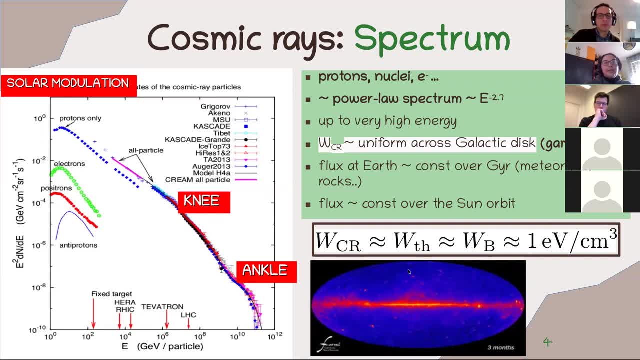 and the magnetic energy density, and it's roughly one electron volt per centimeter cube. This is important because cosmic rays play an active role in the galaxy. It's comparable to other very important parts of the galaxy, so the thermal and magnetic part. 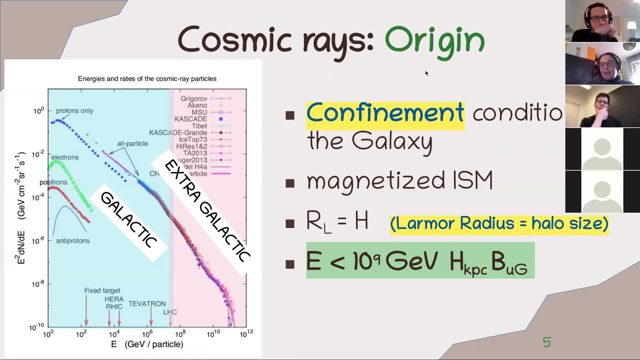 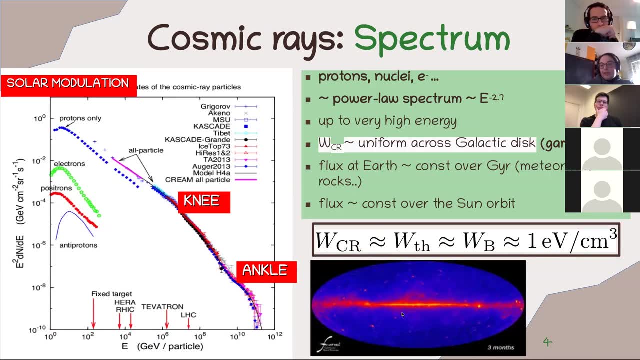 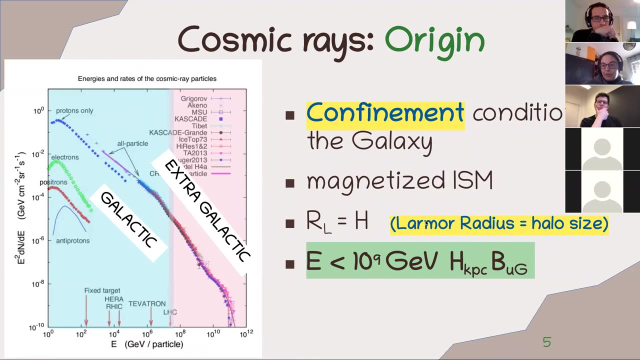 So how do we know that some cosmic rays can be galactic and some must be extragalactic? Well, we know that we have galactic cosmic rays because we see the disk shining in gamma rays, And then we will see that there are confirmations from observation. 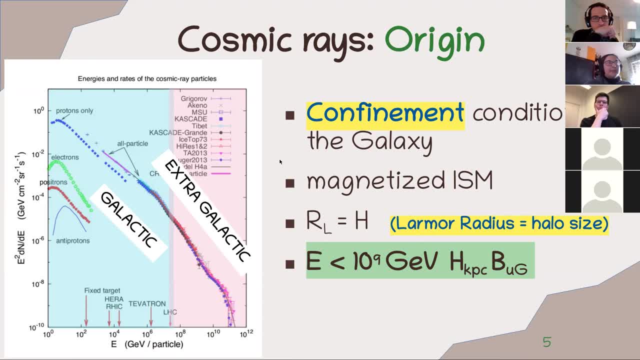 that supernova remnants accelerate cosmic rays, But the more we go up in energy, the less cosmic ray can be confined in the galaxy. Indeed, we have to remember that the interstellar medium is magnetized with a magnetic field of microgauss scale. 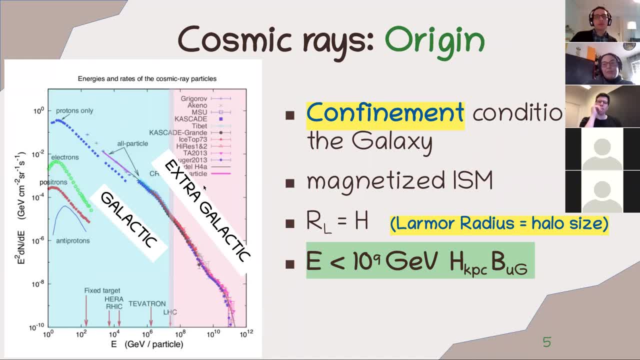 So, in order for cosmic ray to be of galactic origin, they must at least be confined within the galaxy, Otherwise they cannot even be accelerated. And so, if we compare the Larmor radius to the size of the halo of the orbit of Kiloparsec, 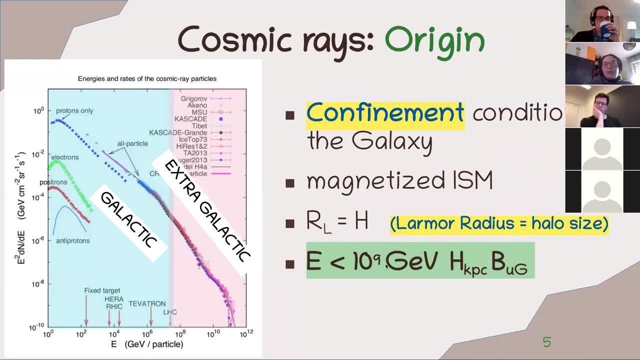 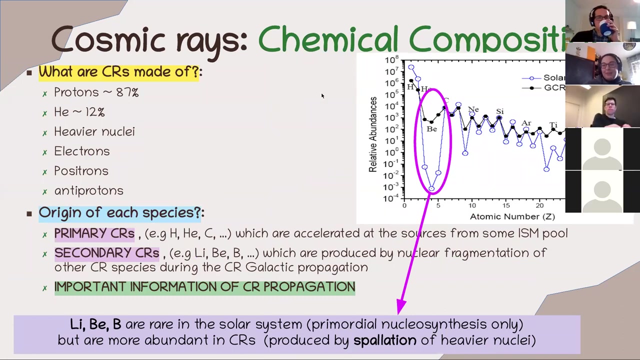 we get a rough information of the energy above which cosmic rays must be extragalactic. Then the specific point of transition is not well known. But this topic is not very relevant for the present analysis because we focus on low energy cosmic rays. Then we go to the main part or the main piece of information that we get. 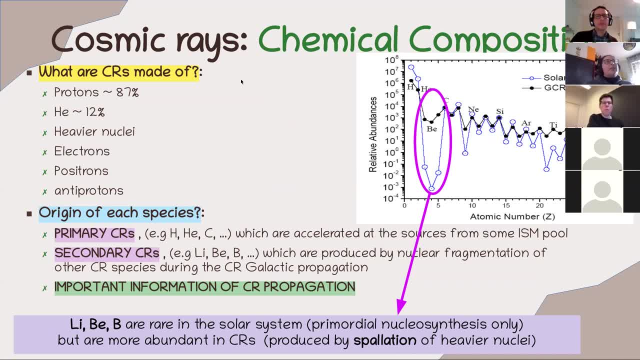 which is related to the chemical composition. So what we see is that cosmic rays are mostly protons and helium, with small amounts of heavier nuclei, electrons, positrons and antiprotons. But nuclei, despite being in small amounts, provide very precious information. 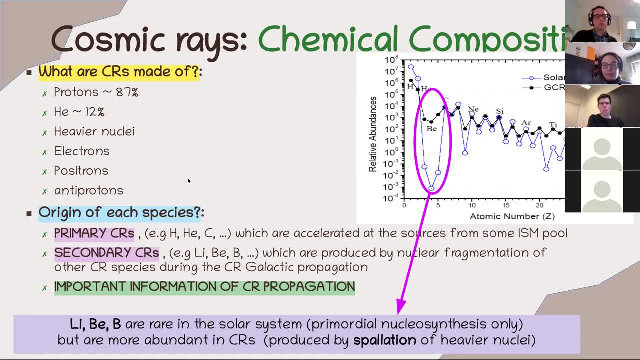 on how cosmic rays are accelerating, They propagate in the galaxy. In fact, there is a very important distinction that we have to make between cosmic ray species. So primary cosmic rays, such as hydrogen, helium and carbon and so on, are species that are likely accelerated by sources and extracted from the ISM pool. 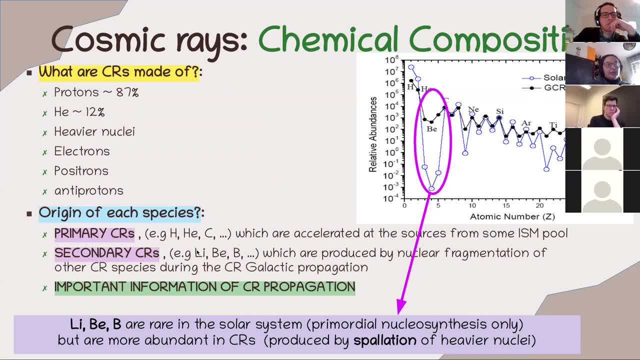 While there are other species, in particular lithium, beryllium and boron, which are of secondary origin. Namely, they are not accelerated directly by sources, but are produced by the nuclear fragmentation of heavier cosmic rays, while they propagate in the interstellar medium. 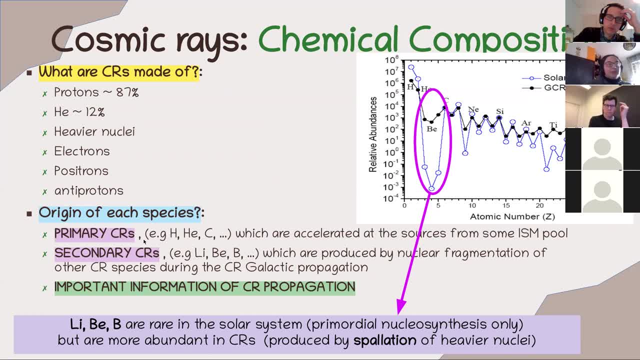 And so if we look at the abundances of these secondary spallation nuclei, we get an important information on how cosmic rays propagate. Why lithium, beryllium and boron are so important Basically because in the normal interstellar medium they would be very rare. 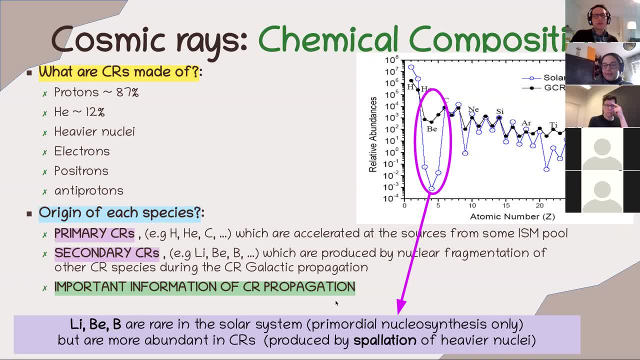 since they are produced in primordial nucleosynthesis and not in starts. So we would expect that if these particles are simply accelerated from the ISM pool, they would be very rare, But instead in cosmic rays they are orders of magnitude more abundant. 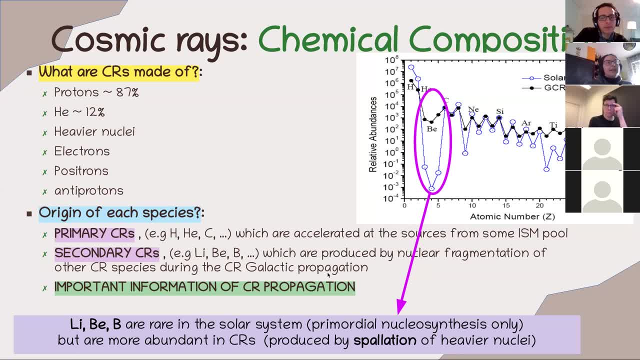 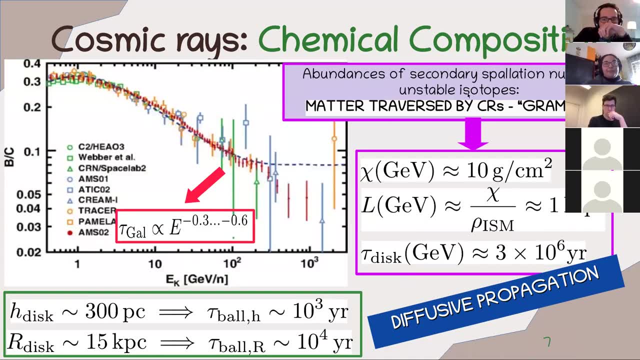 than in the normal interstellar medium, And this is because they are produced by this nuclear fragmentation, And so from the abundances of these secondary spallation nuclei and stable isotopes such as beryllium-10,, we get basically two information. 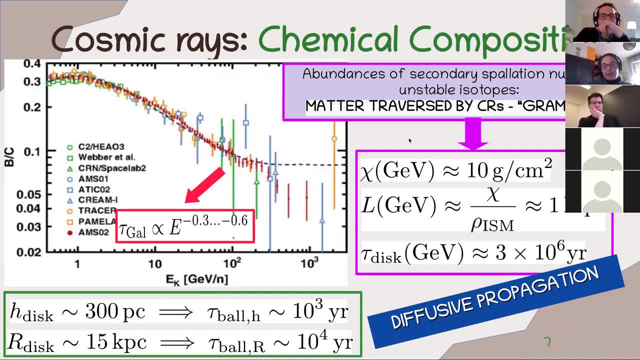 which is the amount of matter, so namely the grammage traversed by cosmic rays during procapagation and the residence time of cosmic rays in the galactic disk. And when we look at the information extracted from this composition, we see that the average distance traversed by cosmic rays at 1 GV. 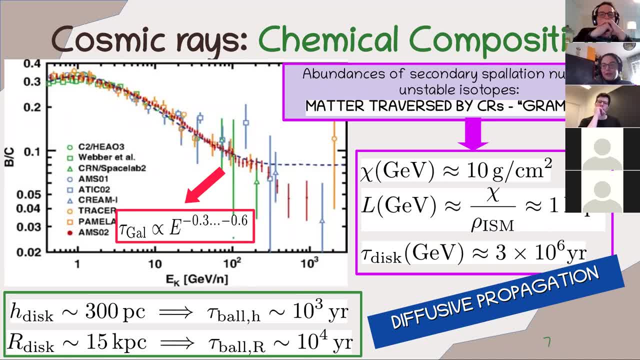 should be of the order of one megaparsec, which is much larger than the typical distances of the galaxy, and the residence time would be of the order of one mega-year or so, And both length and time scale are much larger. on what is the height of the disk or the disk radius. 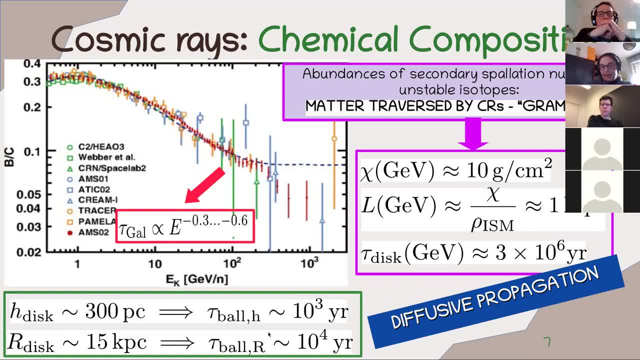 and the time required to cross them ballistically. So this is the main information that we have on the fact that cosmic rays must propagate diffusively in the galaxy And, moreover, if we look at the energy dependent residence time which is provided by the boron over carbon ratio. 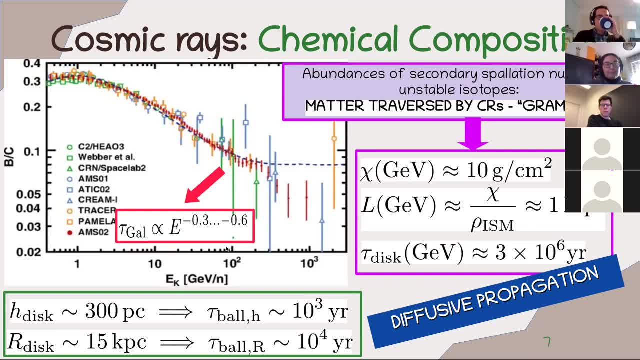 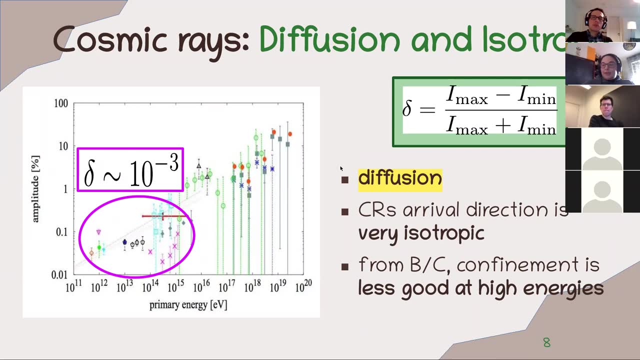 for instance as a function of the kinetic energy, we see that the residence time decreases with the energy, So particles with larger energies are less and less confined. The diffusivity of the propagation is also confirmed by the very small anisotropy of the cosmic ray arrival direction. 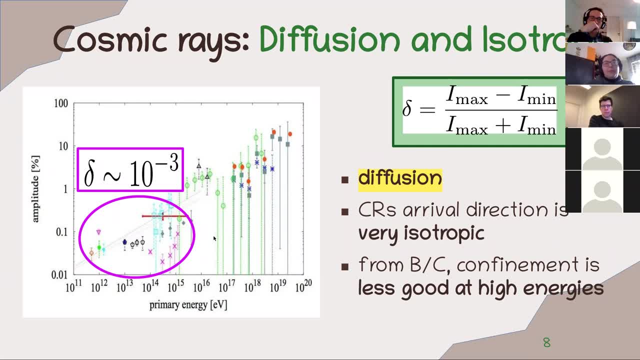 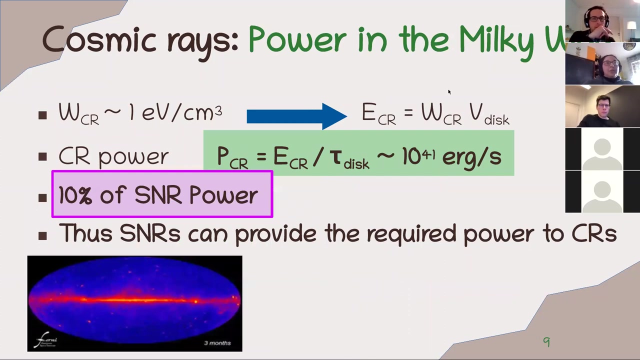 This is problematic if we want to study cosmic rays, because basically we cannot track the source, but we have to investigate the sources in an indirect way, because during the propagation the cosmic ray direction is isotropized. Finally, putting together what we know about the residence time, 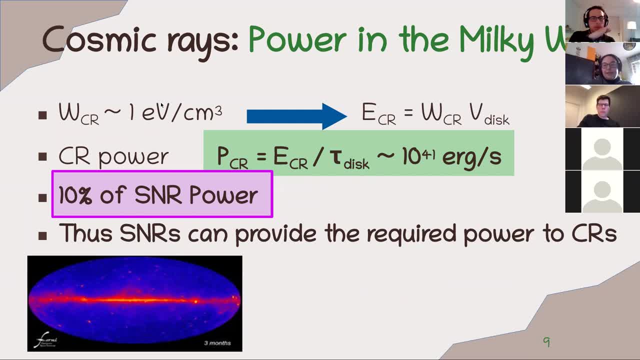 of cosmic rays in the disk and the average density of cosmic rays, we can extract an information on the overall power that sources need to inject into cosmic rays In order to detect what we detect, And this is of the order of 10 to the 41 hertz per second. 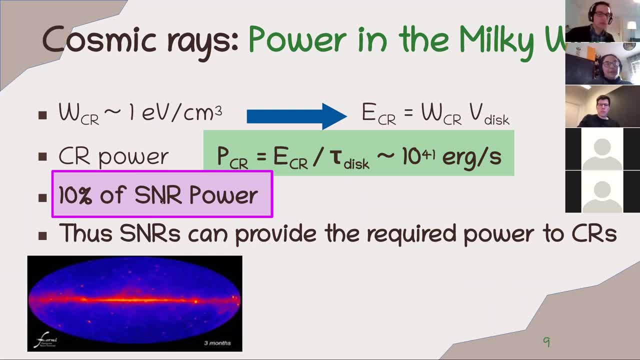 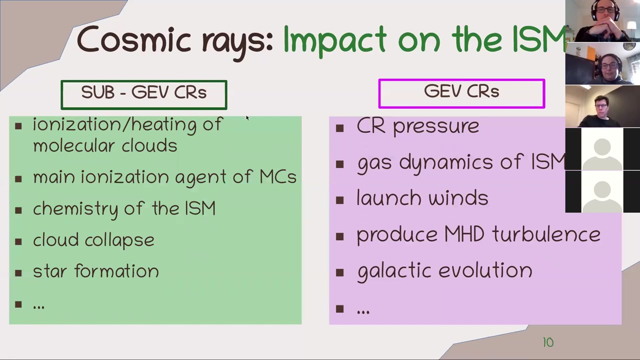 which is roughly 10% of the supernova remnant power. So this energetic argument was the first one put forward several decades ago to start to study supernova remnants as the main source of galactic cosmic rays. Finally, as a remark, it is important to stress that cosmic rays are not only important per se. 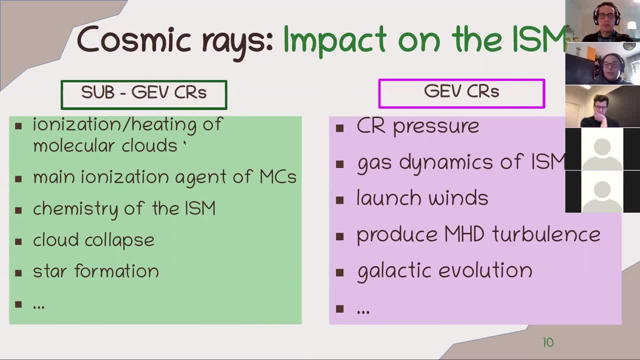 but they play a very important role in the ecology of the galaxy. In fact, in the sub-GV energy domain they provide the main ionization factor of molecular clouds, And namely they basically drive the chemistry of molecular clouds and in general of the interstellar medium. 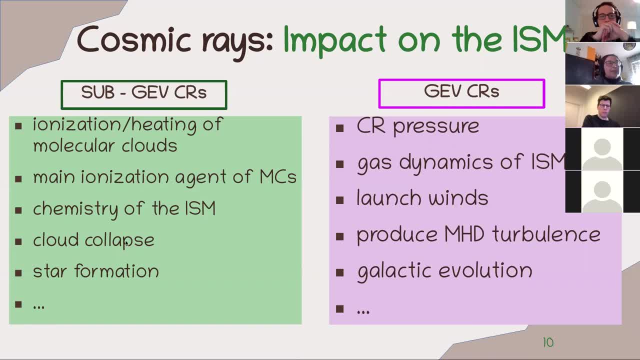 And so, by ionizing the clouds, they change the rate at which they can collapse, And so, finally, they affect the star formation. On the other hand, if we look at the GV energy range, where most of the cosmic ray pressure is present, 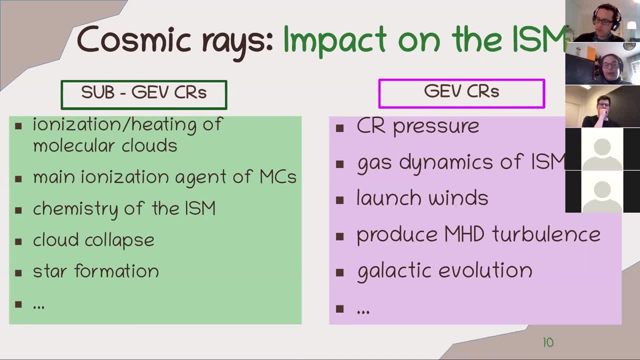 basically, this cosmic ray pressure provides a very important pressure gradient between the disk and the outer halo, is an important force that can affect the gas dynamic of the interstellar medium And, for instance, can launch galactic winds. And launching galactic winds means that also the galactic evolution is affected. 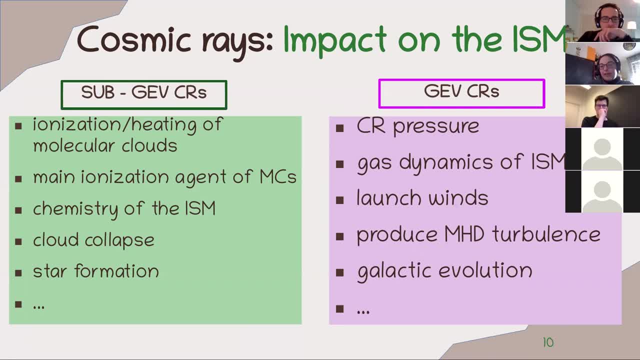 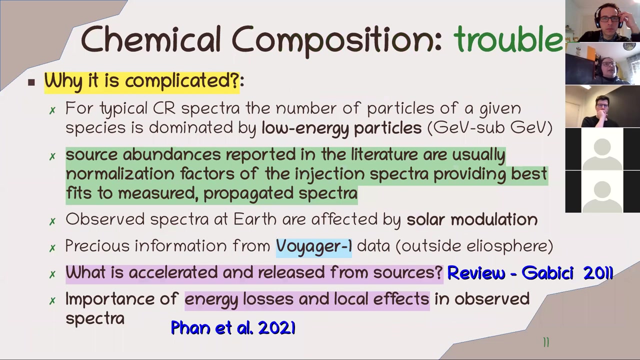 Moreover, cosmic rays are charged particles that stream in the interstellar medium, And so we can have currents that can produce magneto-hydrodynamic turbulence, And so they can also affect the magnetic structure and turbulence of the interstellar medium. So they are active players in the ecology of the galaxy. 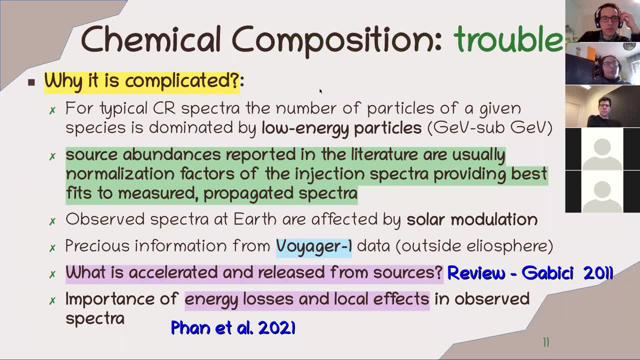 So here is just a recap on why studying the chemical composition is important, but it is also very difficult. So it is important because the main information on where cosmic rays are extracted is hidden in the composition. But it is complicated because, as I said, 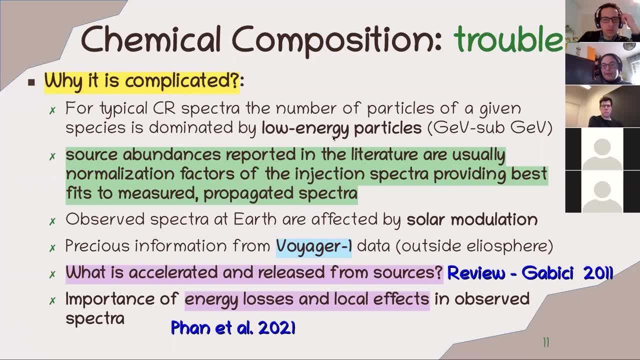 it's the low energy part of the spectrum of cosmic rays that contains the information on the composition, And in this energy range we have much less information due to the fact that, basically, only Voyager can see a spectrum which is not affected by solar modulation. 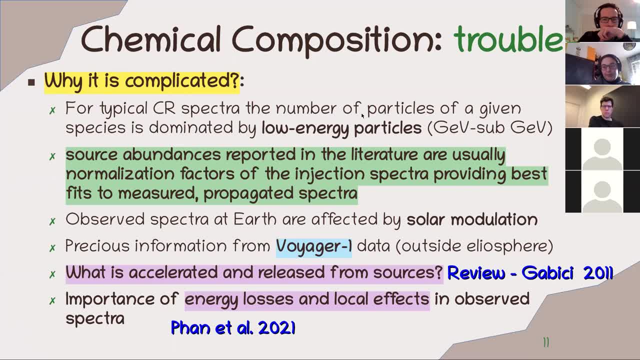 And we have this data since a few years Plus. what we detected is the convolution between the source contribution and the propagation, And we have to disentangle these two contributions in order to understand what is really produced by the sources. And this is not easy because also the propagation. 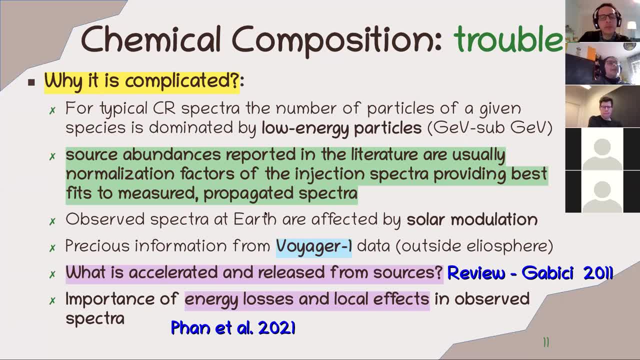 is not so well understood. So, finally, we would need to know very clearly what is accelerated and what is released by supernova remnants and sources. Finally, low energy cosmic rays are much affected by energy losses, which means that also the distance from which we can detect these particles is not arbitrarily long. 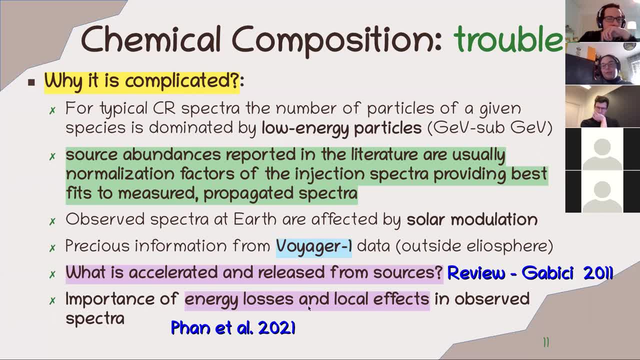 arbitrarily really big, but it could be a few hundred parsecs from the Earth, for instance, depending on the importance of energy losses. And so when we study low energy cosmic rays, also local effects can become important, For instance if we have a recent and nearby source. 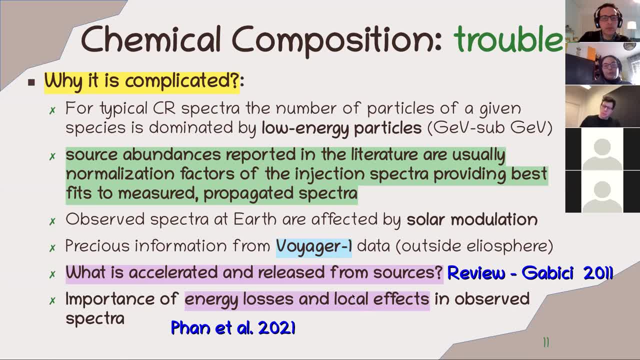 this could affect the composition and the cosmic ray spectrum at low energies much more than the average cosmic ray population. So, Sara, can I ask a question about your previous slide? So you say Voyager has some sensitivity to the composition, but is it just like electrons versus protons? 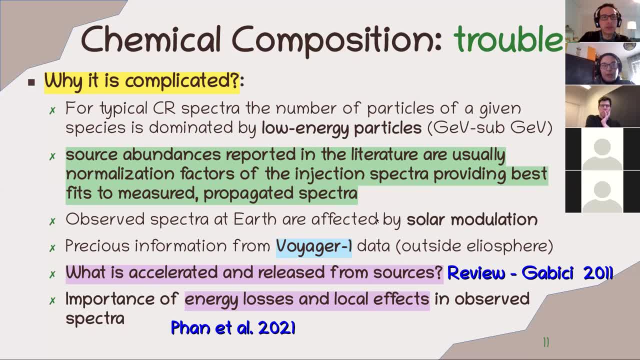 or can it actually tell you what nuclei the cosmic ray is? I don't remember if it had some information of any of the nuclei, But for sure, if it gives some information on protons, we will see that it is important to understand also. 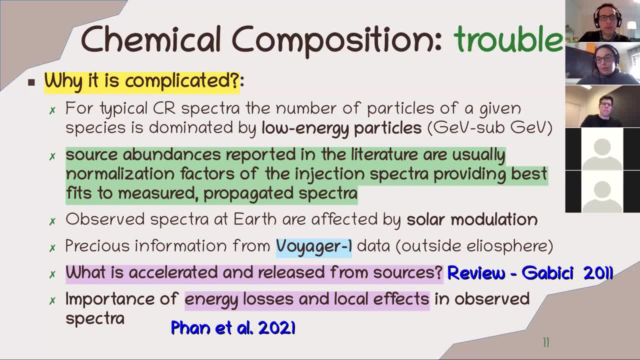 the composition of others, because there is What is important is the composition of one element compared to the others, And there is an issue in particular related to helium and hydrogen, because it seems that they could be underrepresented compared to other species. But this depends a lot on the minimum energy. 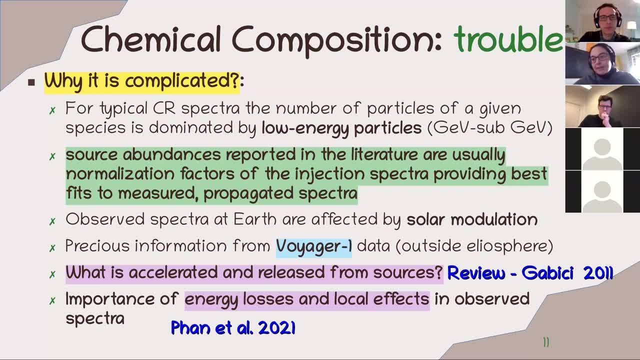 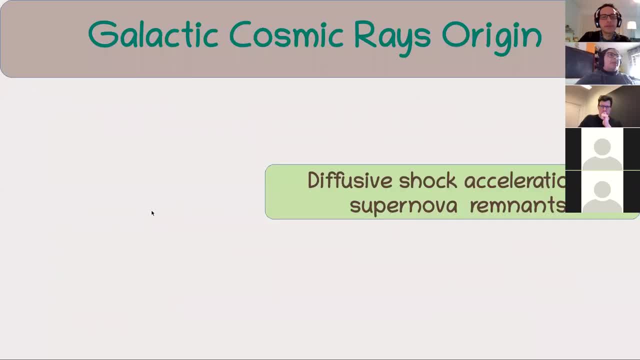 that is in the spectrum, So I will discuss this later. Thank you, Okay, Okay, Here I will just put a few slides to summarize how diffusive shock acceleration is supposed to work And how diffusive shock acceleration treats particle of different species. 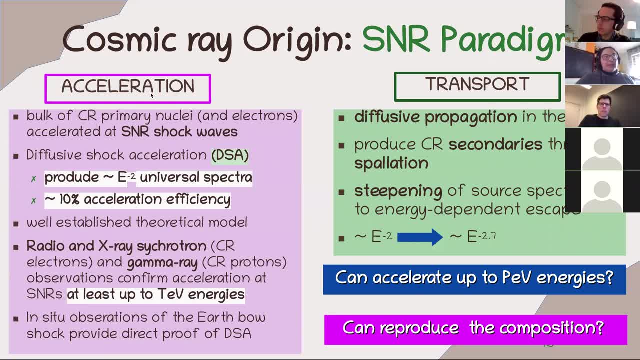 So basically, the supernova remnant paradigm tells us that the bulk of cosmic rays will be mostly accelerated by supernova. remnant shocks And diffusive shock acceleration will produce nearly universal spectra with a power law with 10% of acceleration efficiency, This overall picture is confirmed. 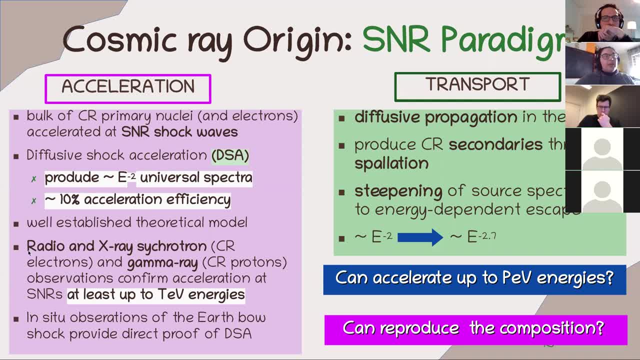 by observation of supernova remnants, because we detect radio and X-rays from the acceleration of electrons, But also if there is some target gas nearby the supernova, for instance a molecular cloud. we can also detect the proton-proton gamma ray. 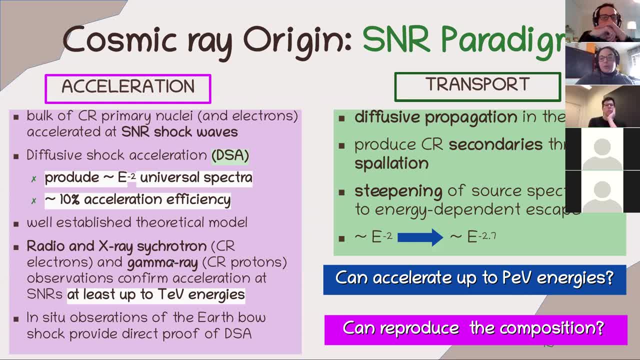 produced by proton-proton interaction, And so we know that cosmic rays can be accelerated up to TVA energies in supernova remnants. Moreover, there have been observations in situ at the Hurt-Bohr shock which proved directly the possibility that diffusive shock acceleration. 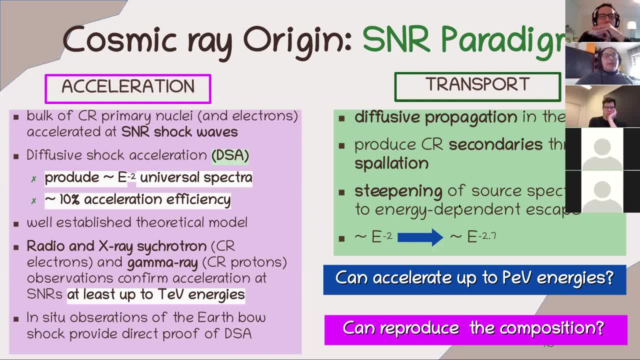 happens really in shocks. Then how can we go from an E2-2 to E2-2.7 spectrum? this will be due through the propagation of cosmic rays, with an energy-dependent escape, with higher energy particles which are released earlier. Okay, 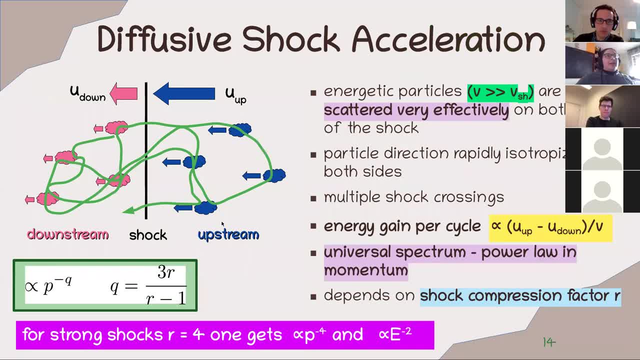 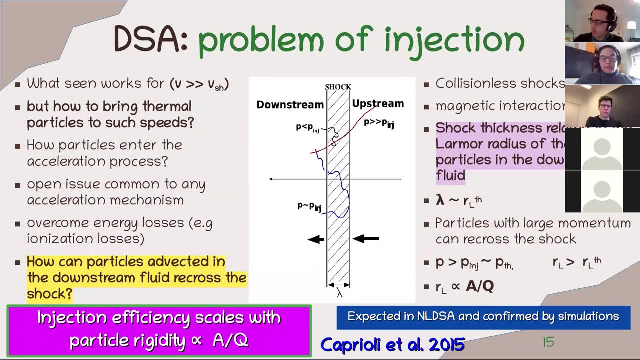 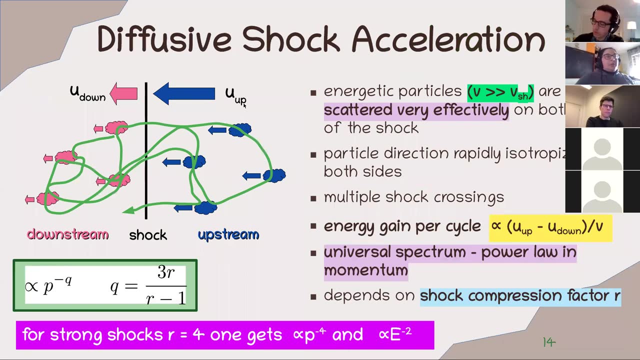 this was just a recap of the scenario, How it is supposed to work: diffusive shock acceleration. Basically, let us suppose that we are in the rest frame of the shock which is here. draw in this picture is this black line And we would see. 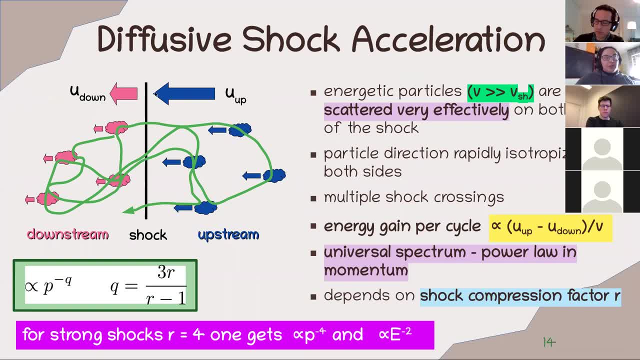 the upstream fluid entering the shock with a given speed And the fluid in the downstream is slowed down and compressed and heated, Then there will be magnetic inhomogeneity moving with the upstream and downstream fluid that can scatter cosmic rays. So the basic hypothesis. 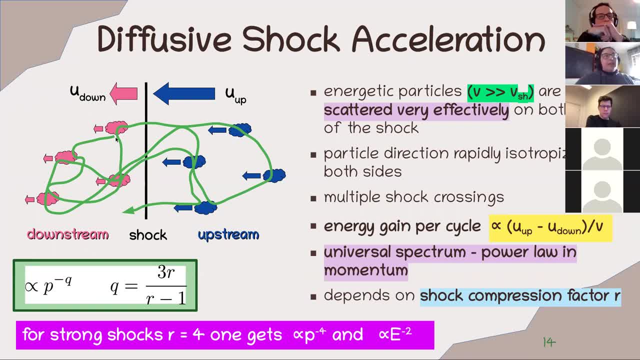 of diffusive shock acceleration is that the scattering in this magnetic inhomogeneity is so strong that when particles cross the shock from one side to the other, particles are immediately isotropized And so they can recross the shock. This is true. 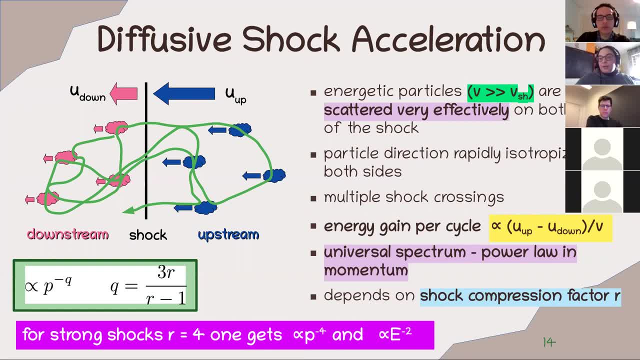 as soon as the velocity of the particle is much larger than the shock velocity. So when this condition is satisfied, basically particles can come from upstream to downstream and are isotropized in each rest frame, And so there will be an energy gain. 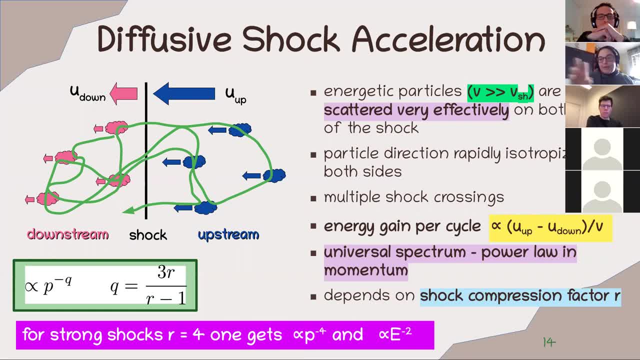 due to the fact that the bulk of the fluid velocity is different between upstream and downstream And there is an energy gain per cycle which will depend on the relative velocity between upstream and downstream fluid. So the interesting part of this scenario is that it doesn't really matter. 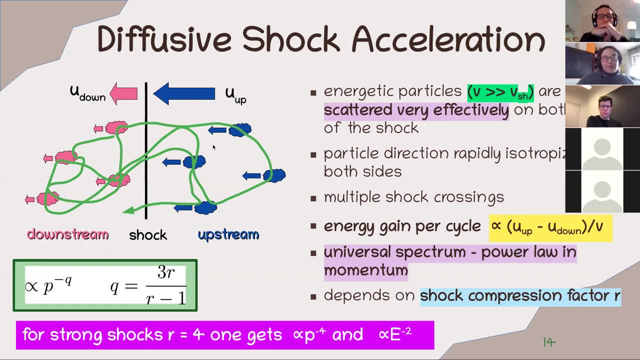 the way in which diffusion works at these scattering centers. The important point is that there must be diffusion. If this is the case, basically we get a power law in momentum for accelerated particles, which only depends on the compression factor at the shock. 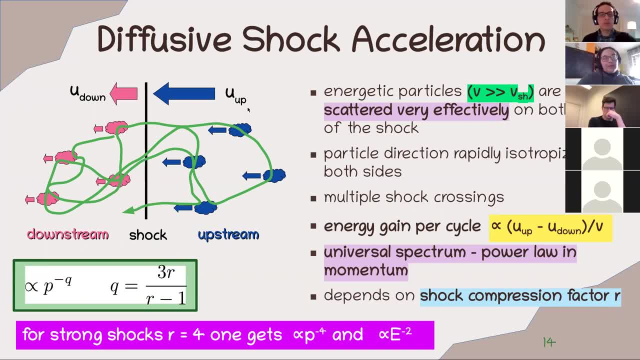 So namely the ratio between the velocity upstream and downstream. So for strong shocks the compression factor is 4.. And so we would get a momentum spectrum to P2-4, which, when we look at the energy dependence, 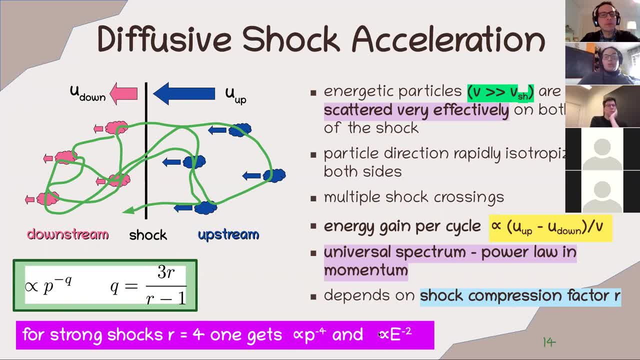 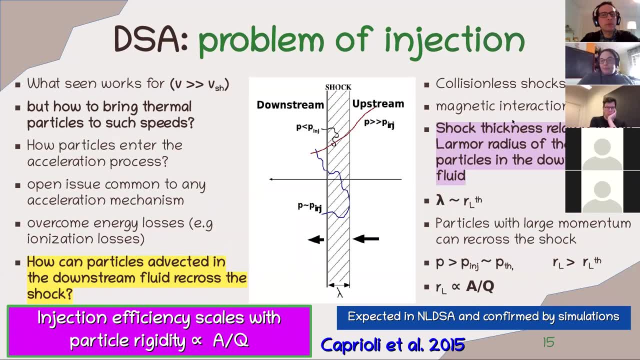 is E2-2.. What is the problem with this picture? It is that, basically, we assumed that the velocity is already equal to E2-2.. So we have to assume that the velocity is already equal to E2-2.. 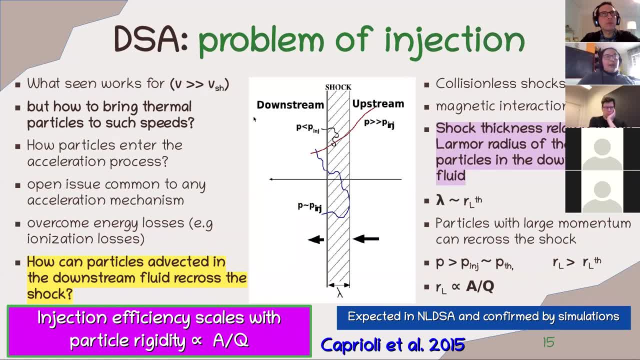 So we assume that the velocity is already much larger than the shock speed. But how particles are taken from the thermal bath and reach enough energy to enter this acceleration process? This is a serious problem of any possible acceleration mechanism And it is not. 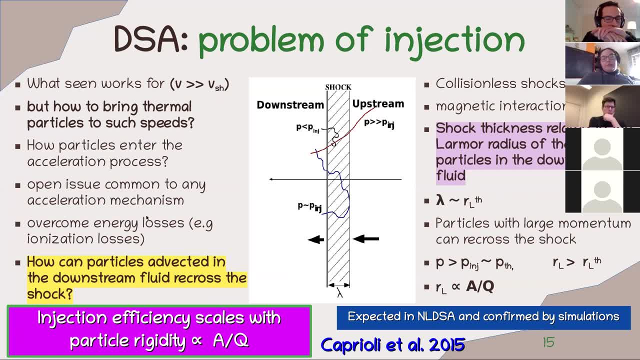 well understood how injection works. So there are two problems related to injection. First of all, at the shock, how to reach the situation of velocity of the particle larger than the shock speed. The other problem is that at low energies, energy losses. 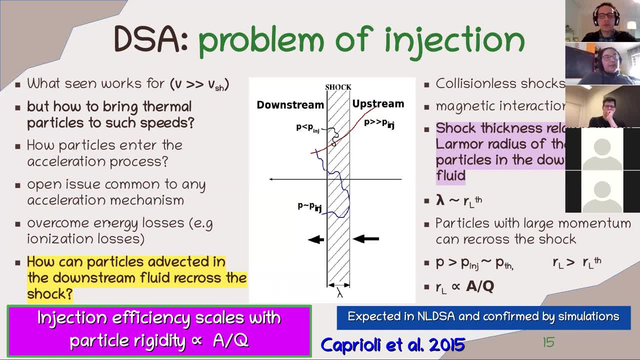 are very important, in particular ionization and Coulomb losses, And so if the acceleration rate in this regime is not large enough, the particle is subjected downstream of the shock before being able to recross the shock. So you have to imagine. 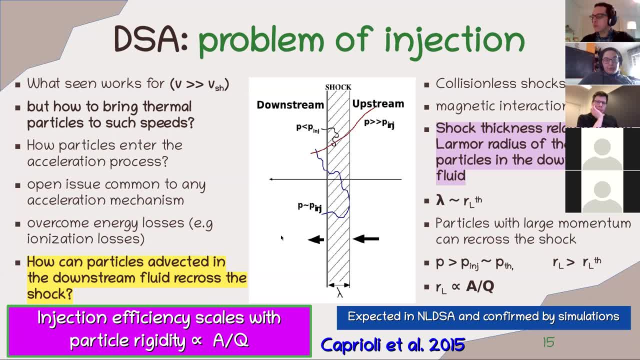 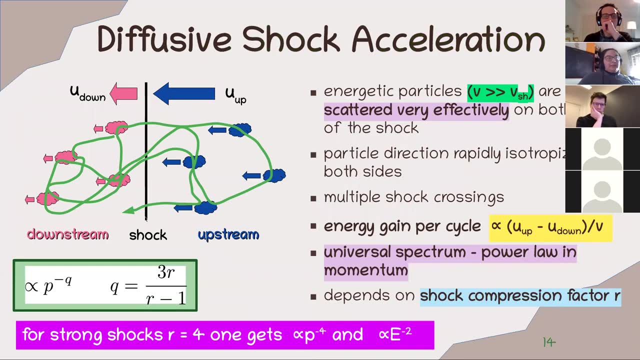 that a particle that crosses the shock. here there is the fluid that is pushing away from the shock in the downstream, And so a particle must be able to recross in order to start the shock as a sharp discontinuity. But in reality, 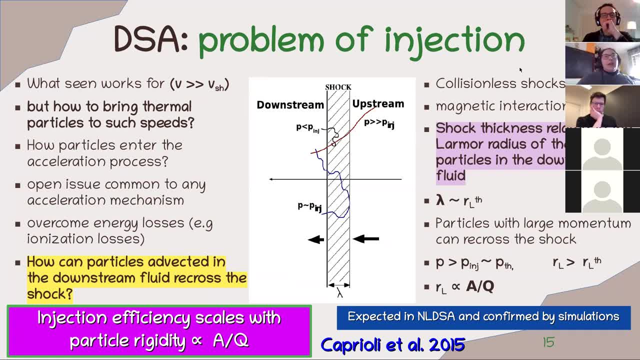 it is not like that, because the shock has a thickness, And since in the interstellar medium collisions are not so frequent because the gas is diluted, the presence of the shocks are mediated by nuclear, by magnetic interactions, And so it is related to the 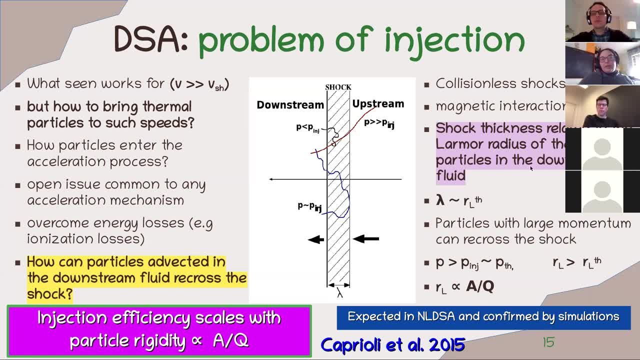 thermal radius of the thermal particles. And so we have this thing that thickness of the shock is roughly the radius of the thermal particles, And so a particle in the thermal tail which has enough thickness without being pushed the way downstream, And so 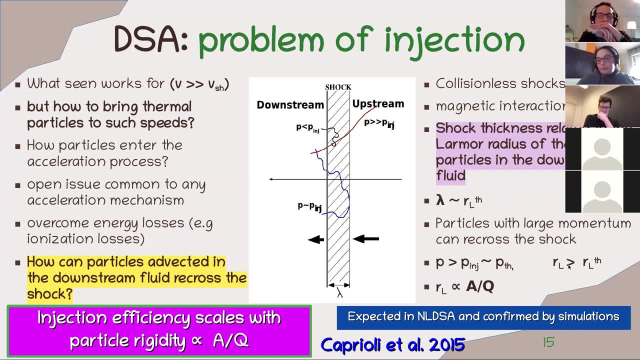 basically, the radius of such particle should be larger than the average radius of the thermal plasma, And so only a tail of this particle could be entered: the acceleration, namely the mass over charge ratio. So what is expected in this scenario is that 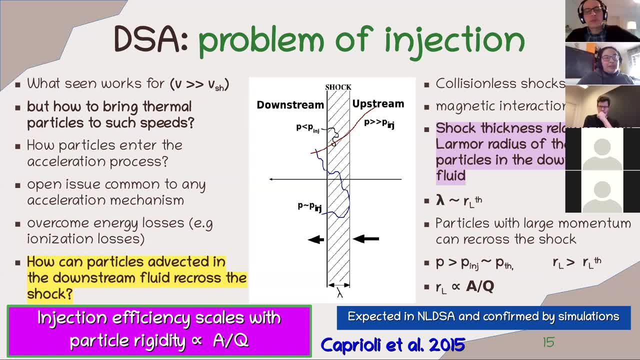 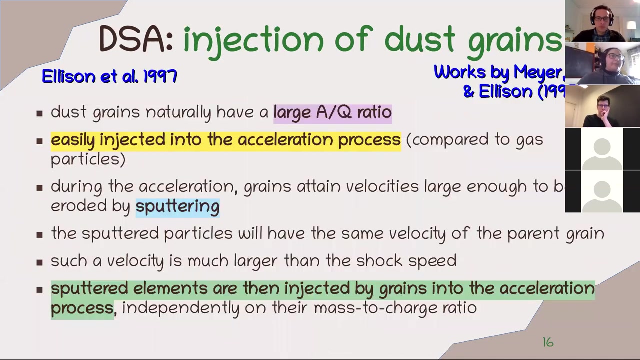 the injection efficiency will scale as the particle rigidity, namely on the mass over charge ratio. So this is expected and somehow it is confirmed by simulations. So there are some simulations that at least confirm this important scaling. This is important because we will 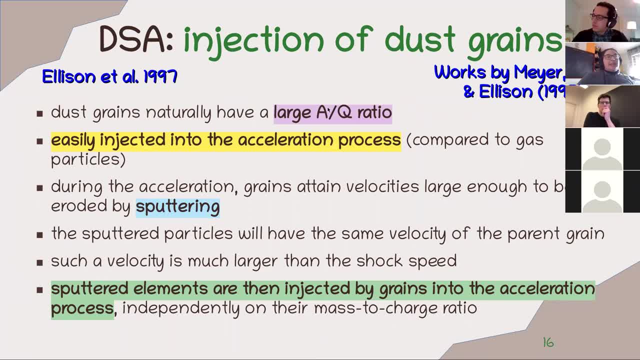 use this scaling in the remaining of the talk. But then so we said that the mass over charge ratio is very large because we can see the mass over charge ratio is very large because the mass over charge ratio is very large because we can see. 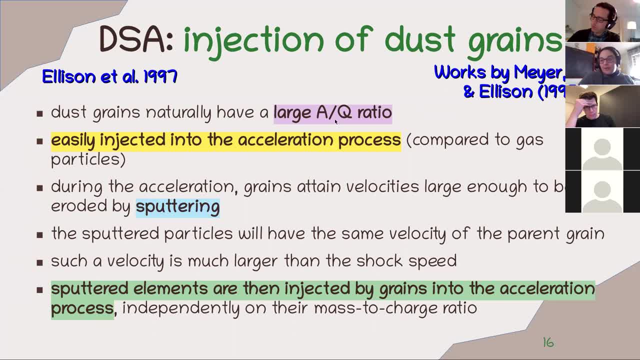 the mass over charge ratio, because we have some ionization of the dust grain but the mass is very large. So we can imagine this kind of mega particles as this dust grains as particles with naturally larger, large radius, and so they will be very large, but at 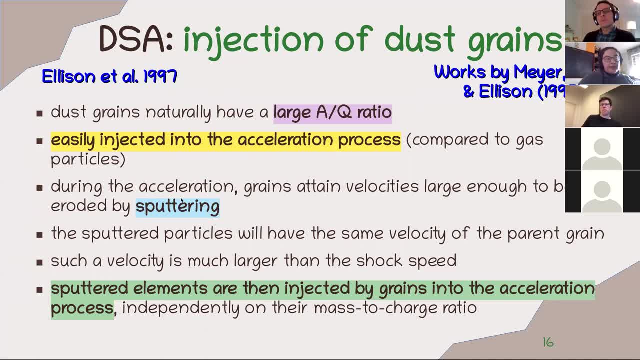 certain point this causes the, the dust grain to be destroyed by the so-called sputtering in the background, plasma. but at this point particles that were locked in the dust grains are released and they have the same velocity of the dust grain, but now they are pre-accelerated. 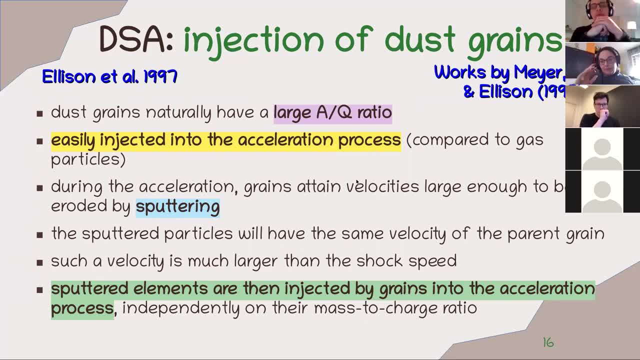 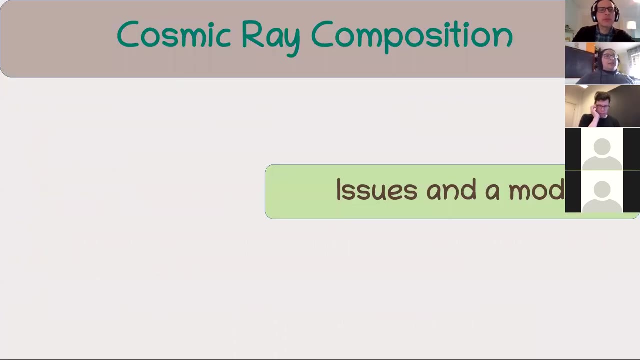 while they are still in the dust grain. and so if we have, if we keep this mechanism in mind, basically we can see that we expect that refractory elements, so the one locked in dust grains, are injected much more quickly. so let's go to the actual study that 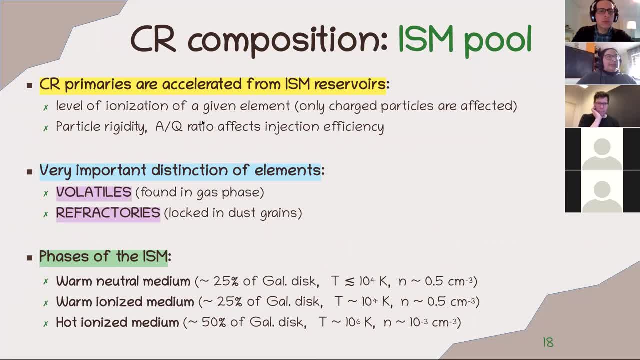 we performed and let's start with a brief recap on what is important for decomposition. so we look at cosmic ray primaries. so we want particles that are directly accelerated in the source, and we know that the injection of particles in the acceleration process will depend a lot on the 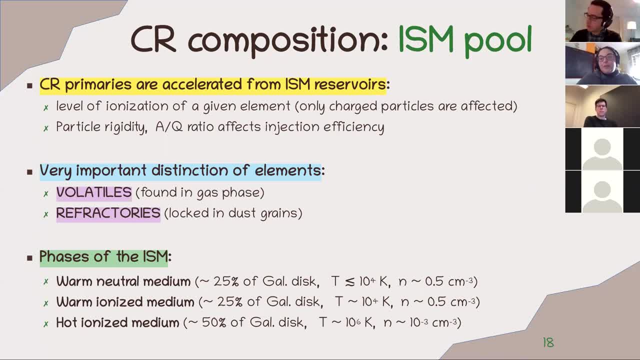 mass overcharge ratio of the particles, and this obviously will depend on the interstellar medium phase, because if the in this, in a specific, there is the important distinction between volatiles, so elements in gas phase and refractories, that will be injected much, much easily compared. 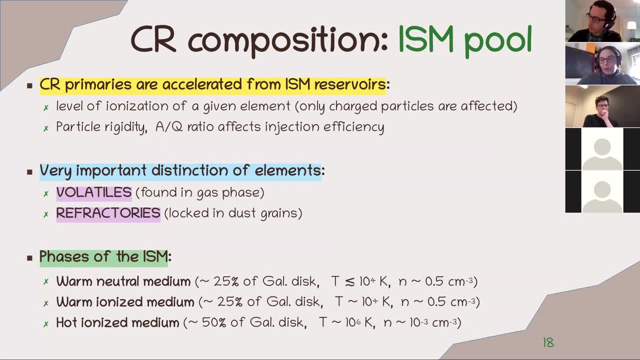 to volatiles. and then we have to look at the interstellar medium phases, which are more interesting, because this is mainly made of warm, neutral and warm ionized medium with a density of roughly one particle per centimeters cube and with a temperature which is somehow 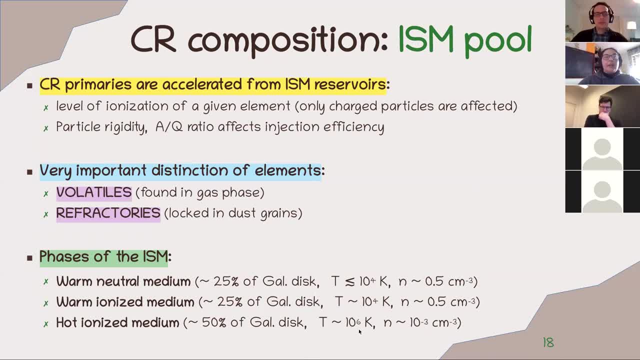 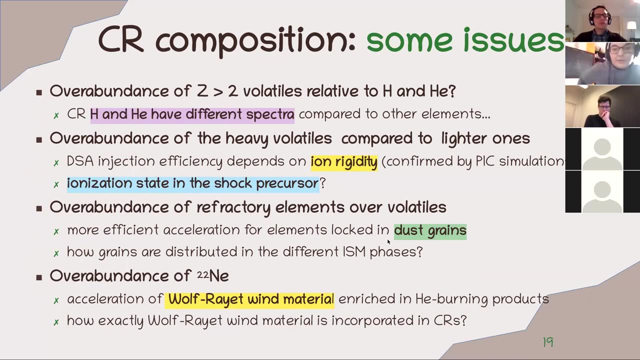 around 10 to the fourth kelvin, uh medium and relatively dilute, with 10 to minus three centimeter particles per centimeter cube. so what are the issues that we should address when we look at the composition? so then i will explain in detail each of. 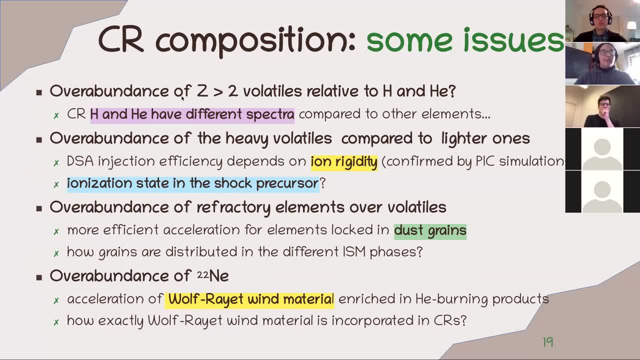 these issues. so, first of all, we see that there is an overabundance of not heavy volatiles, so for zeta larger than two relative to hydrogen and helium. why i say that? maybe there is an overabundance because we have a slightly different from. 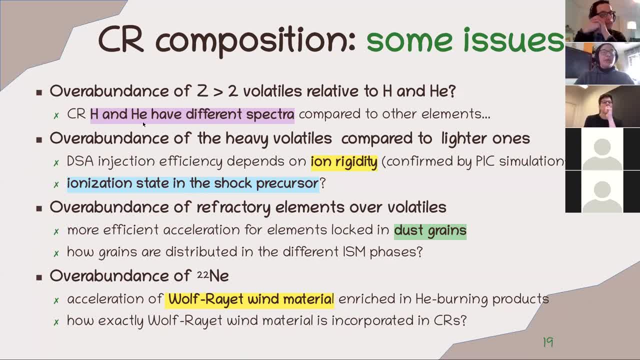 these other species and for such elements, so for hydrogen and helium, the number of particles, so the composition, depends a lot on the minimum energy, and if we use this as minimum energy there is an overabundance, but if we assume that the spectrum goes even below this, 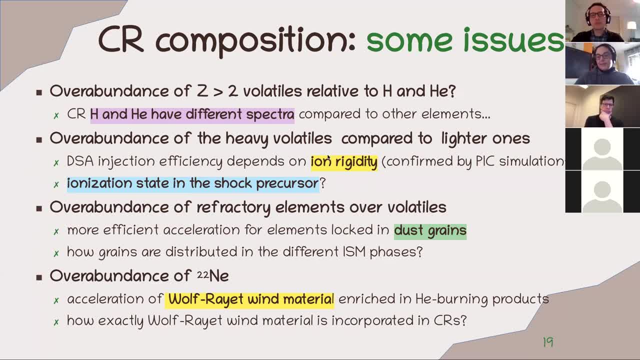 three me, the overabundance is not there. then there is an overabundance of refractories compared to volatiles, and this is due basically to the most more efficient acceleration of dust grains. and finally, there is an overabundance of neon 22. if 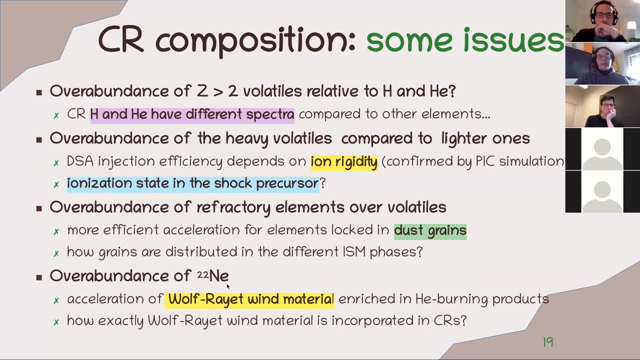 some wolf wolf right here. wind material which is enriched in the neon 22 is also accelerated. the problem is is also to establish how this acceleration of dust grains also depends on the, on the size of the dust grains right and or maybe, maybe the masses is a. 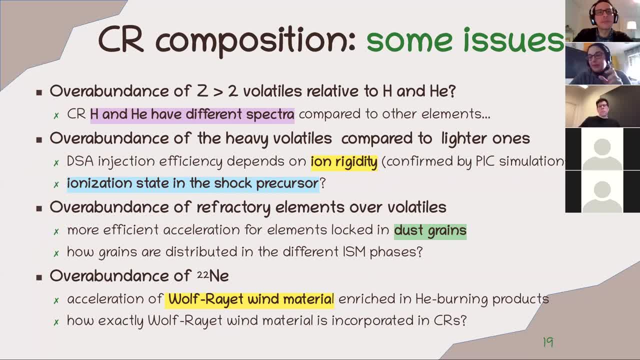 better way to say it. well, the point is that, since the ionization level when we look at the spattering, so this can, this can have an impact, but it has not really. it has not been well understood, also because we will see that they are injected much. 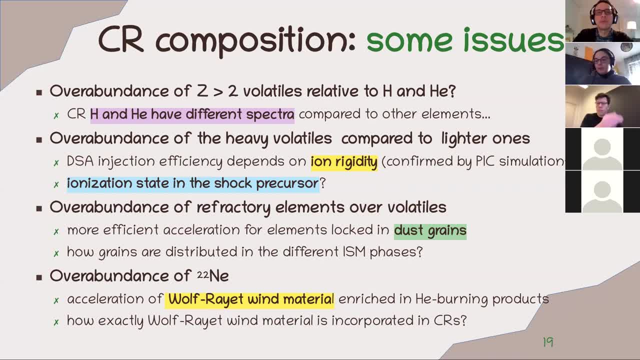 more easily, but the point is that as soon as the grain is injected, then the spattered particles will be injected, and so, finally, probably the exact initial size etc will not be shown in a while. that was, that was connected to my question, actually. so the follow-up. 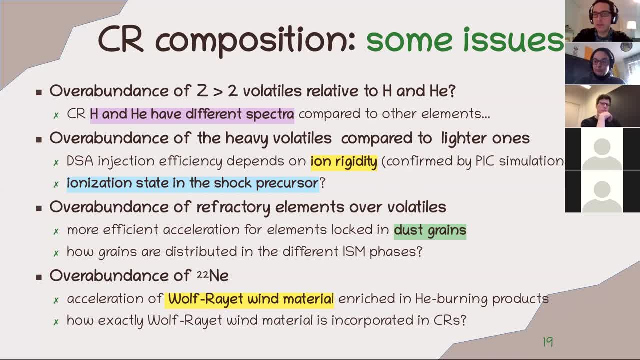 is: these dust grains are those injected by the supernova that gave rise to the supernova remnant, or are those dust grains in the interstellar medium from the interstellar medium, for instance in super bubbles? it is not clear whether they are present, whether they are. 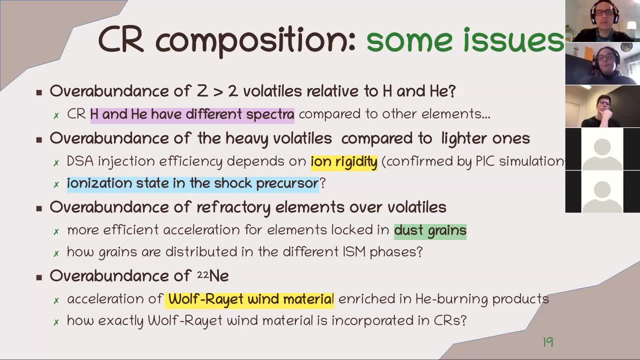 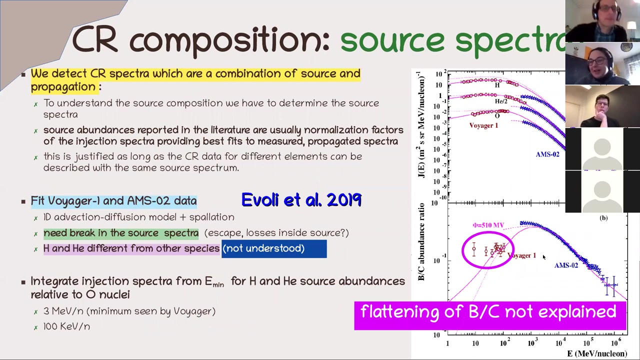 destroyed by the multiple explosions or whether they are in this outer skin of the supernova. so I mean, I do not know the actual observational details and the references to where to look, but unfortunately it's not well known. thank So sorry. I don't know why. there was a moment in which I forgot. 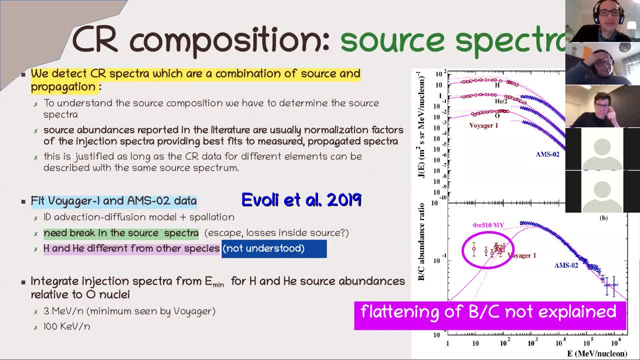 OK, so, OK. so now I will go to some details in every of these points that they have been putting forward for the composition. So the first one is: how do we disentangle? So what are the data for the abundances that we are really using? 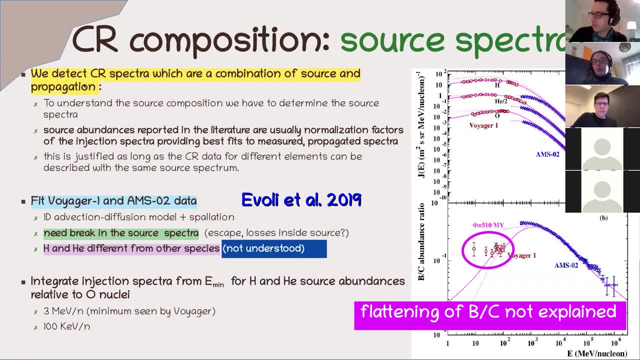 This is an important point because, as I said, we detect a combination of sources and propagation And so, and usually in the literature, the abundances data are basically given as follows: So people take some sort of spectra that, once propagated, provide good fit to the propagated spectra. 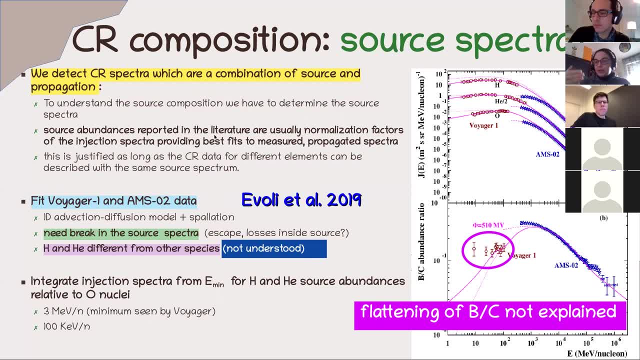 And then the abundances, But the abundances are just normalization factors of the injection of this injection spectra. Unfortunately, this does not work if the injection spectrum is different from the four different species, And this is exactly the problem that we have for hydrogen and helium. 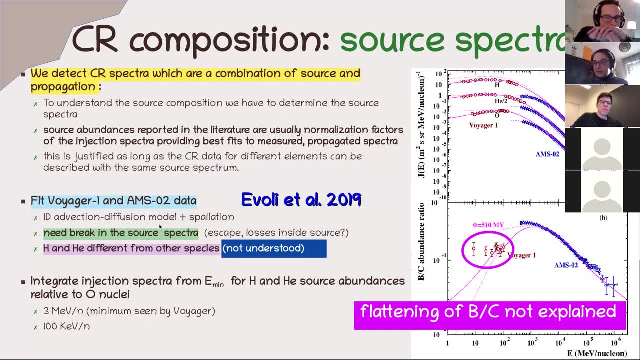 Indeed what we confirm this problem, because what we did was to take Voyager data And IMS data And to extract the source spectrum Using a propagation spectrum, a propagation model which was provided by Evo Lietal, in which we adopt an advection diffusive model plus spallation for mostly primary cosmic rays. 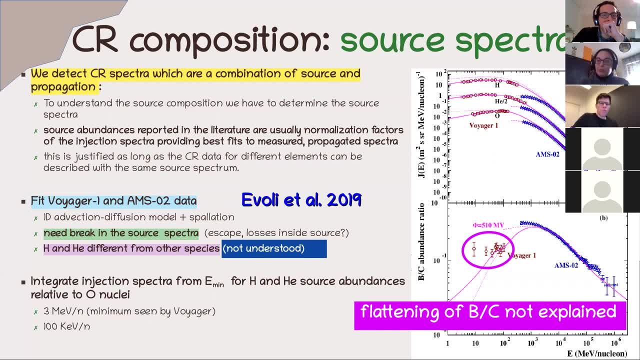 So from this propagation model we can extract What is the injection spectrum at sources And which is then propagated and gives what we observe. And when we play this game, what we find is that basically we need breaks in the source spectra And such breaks are not in the same position as energy per nucleon for every species. 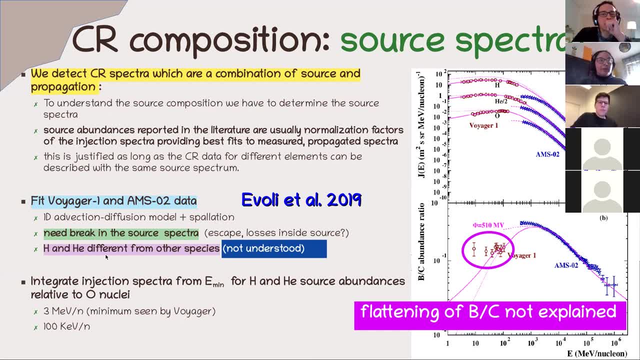 And in particular hydrogen and helium, have different source spectra compared to other volatiles. Why it is so, It is absolutely not understood. This is something that should be addressed in the future. So so far I have not seen in the literature no convincing explanation. 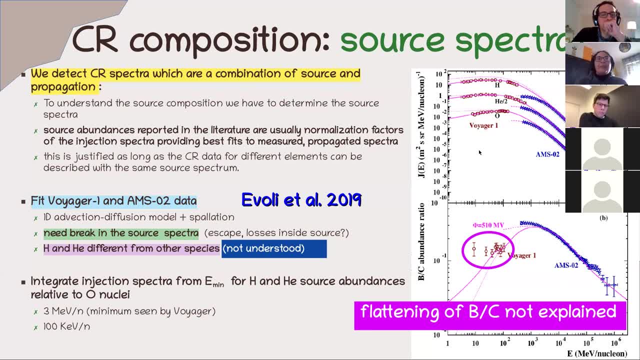 But so this is what we get. Moreover, there is another issue which is related to the propagation. So when we look at this data for the boron over carbon ratio, we see that in the low energy part, so below a few hundred MeV, the boron over carbon ratio drops and becomes flat. 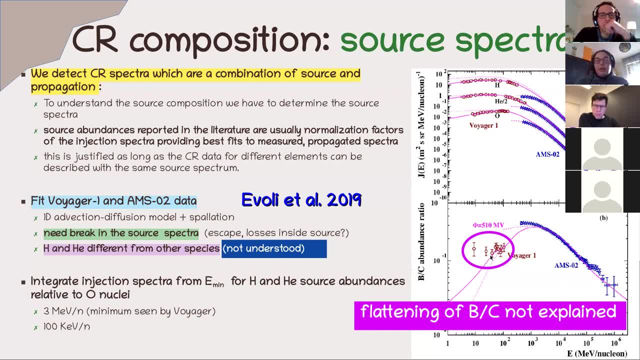 Also this is not understood. So here there are two problems. So from the one end the propagation of low energy cosmic rays. This is not understood, And so it will be more difficult to extract correctly the source spectra, And this is a general problem. 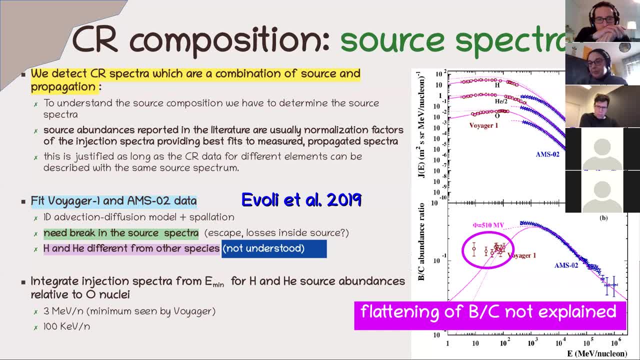 And plus the source spectra that we are able to extract somehow show this difference of helium, hydrogen, hydrogen helium and other nuclei, And And And the problem that with the source spectra that we get for these two elements, The composition really depends on the minimum energy, which is not known because the data Voyager arrive up to 3 MeV per nucleon. 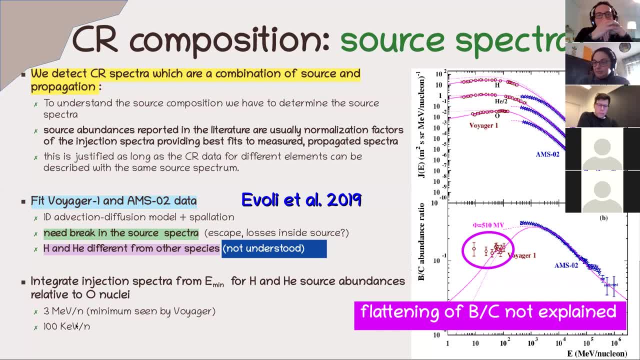 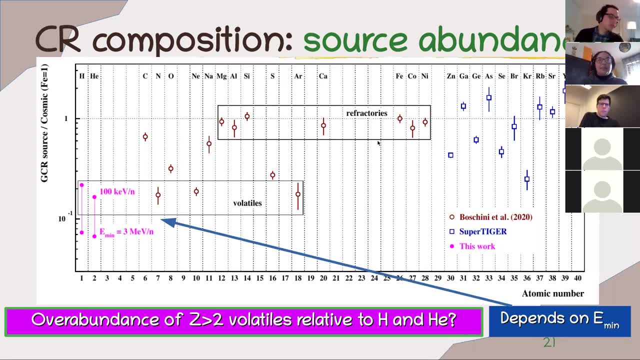 But if the spectrum extends for smaller energies, the number of particles would be much different, And so this is what we get. And so these abundances have been extracted by previous works of Bruce Kinnear from Super Tiger, And so we have here hydrogen helium, compared to light volatiles such as nitrogen carbon, etc. 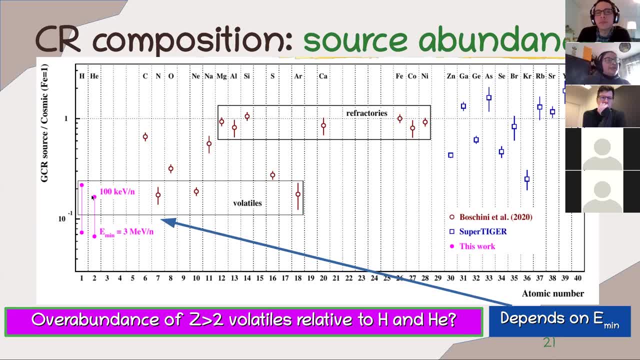 Oxygen And We see that if we integrate the source spectrum starting from 3 MeV per nucleon, we see an overabundance. So these volatiles will be more abundant than hydrogen and helium. But if we integrate starting from 1 KeV per nucleon, there will be no overabundance. 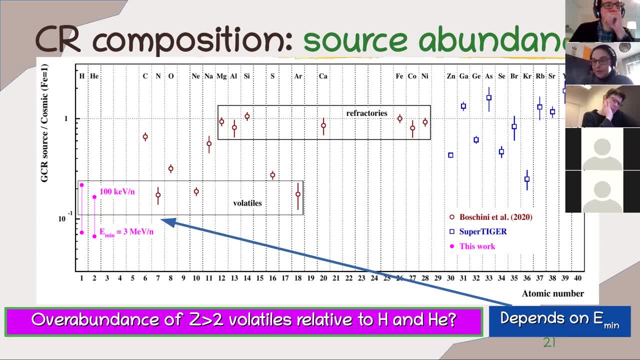 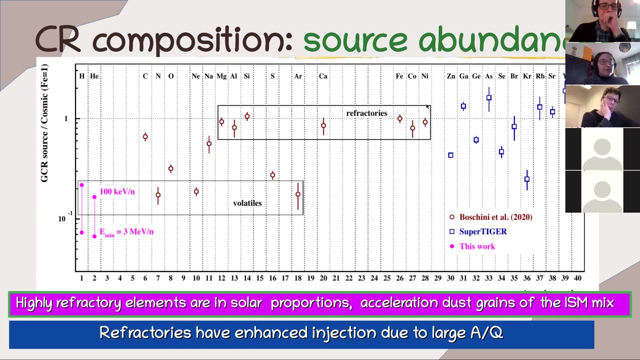 So this is something that, unfortunately, we do not have an explanation for why it is so And, as I said, this should be addressed in the future. Then, if we look at the refractories you see here, for instance, we clearly see that, compared to the volatiles, they are much more abundant. 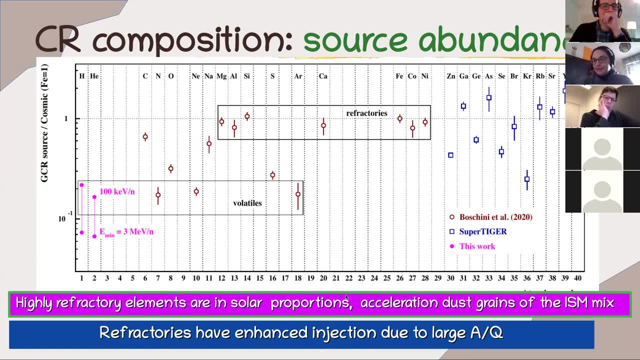 And this can be explained by this dust grain acceleration. basically, This idea is not new, So that's why I said that. So that's why I said that. So dust grain acceleration was put forward in 97 by several authors And it seems to work well, because we clearly see a difference in abundance from refractories to volatiles. 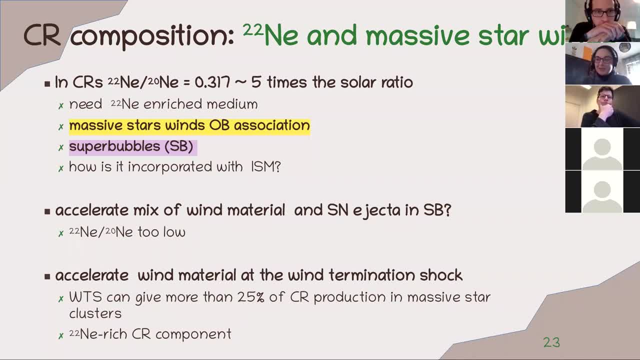 I'm sorry. I know that this matter of these things of composition is very detailed And if something is not clear, please feel free to ask because I understand. I understand that there is a lot of information in there And if something is not clear, please feel free to ask, because I understand. 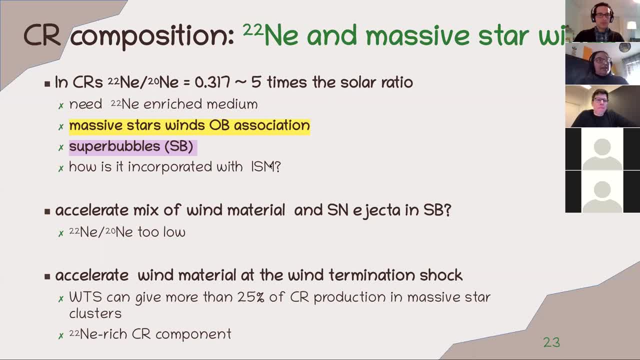 And if something is not clear, please feel free to ask because I understand. Okay, Then again we look at neon 22. And in cosmic ray we see that the ratio between neon 20 and neon 22, it's roughly a factor of five more than the solar ratio. 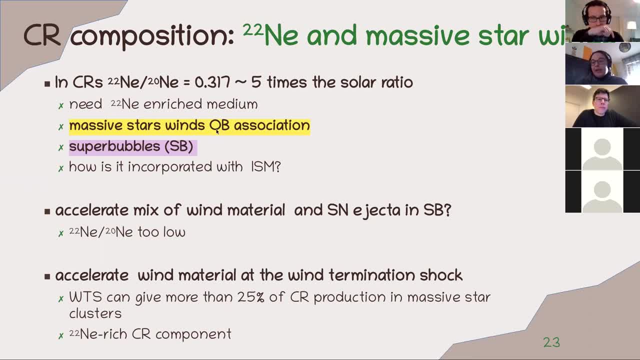 And the only way in which we can get this overabundance is somehow the material. And the only way in which we can get this overabundance is somehow the material. And the only way in which we can get this overabundance is somehow the material. 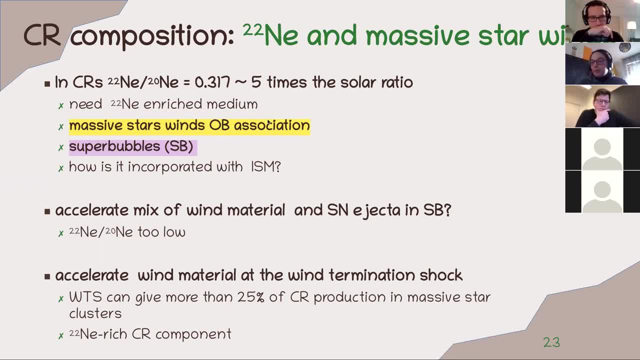 From massive star winds. you know, the association is incorporated in cosmic rays And this material is mainly finding supernova in super bubbles because this massive star winds and repeated supernova explosions excavate the super bubble. But how this material is incorporated is not clear. 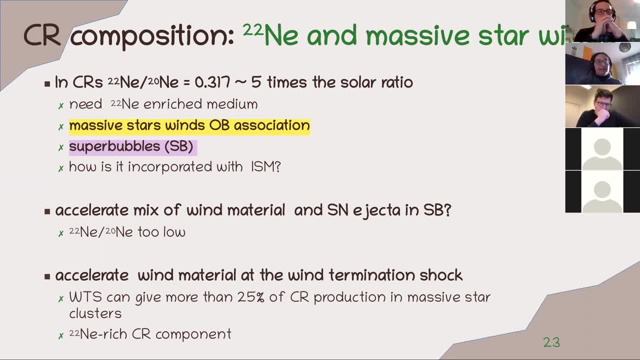 Indeed, in the literature there have been two hypotheses basically for this neon 22 anomaly, Which is that one is that the wind material is deposited within super bubbles and the mix with the normal interstellar medium And then supernova remnants accelerate a mixture of this mixture. 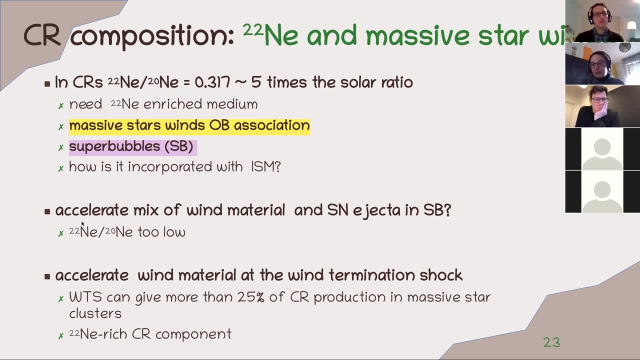 However, in this scenario the neon 22 ratio would be too low. Another possibility is that acceleration happens Directly at the termination of shock of the massive star wind, and in this case it is possible to reproduce the new 22 enrichment. 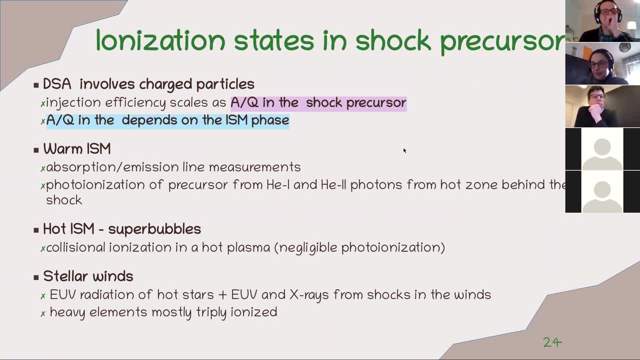 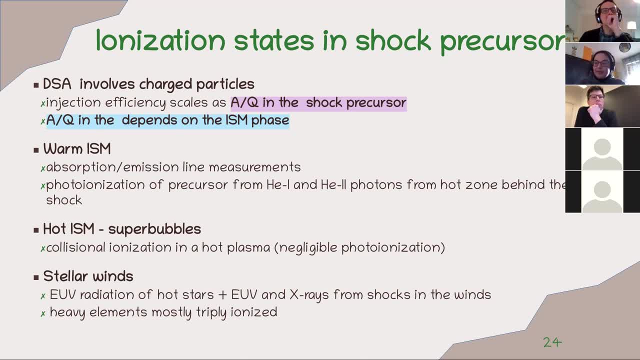 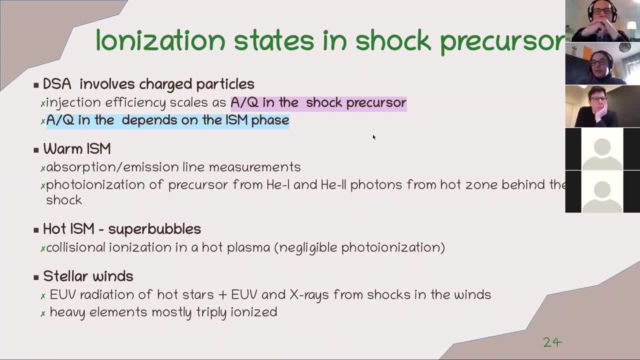 So This was quite complicated because for each ISM phase the ionization level depends on a lot of factors. I will just quote the main points depending on the ISM phase. So basically, in the warm interstellar medium there are absorption and emission line measurements that show that. 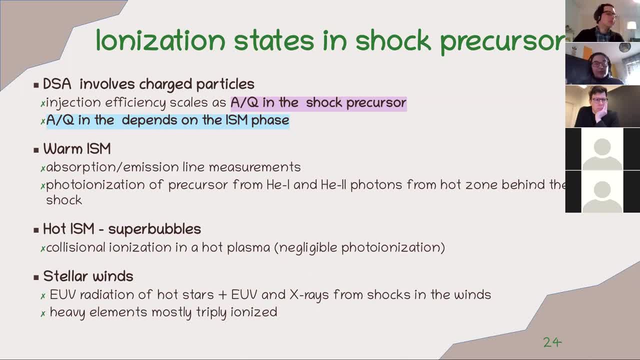 The precursor in the shock can be photoionized due to photons from helium that are produced in the hot zone behind the shock. Instead, when we look at the hot ionized medium of super bubbles, photoionization is negligible, but we have the collisional ionization due to the presence of the hot plasma. 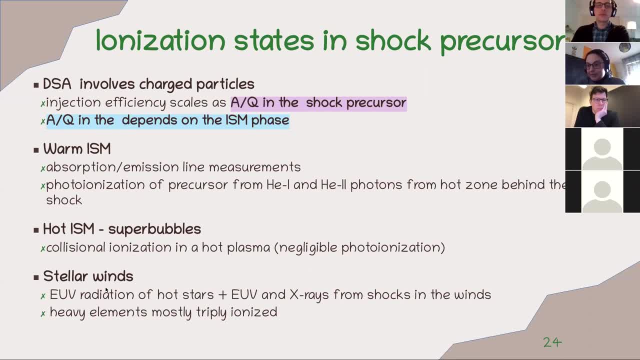 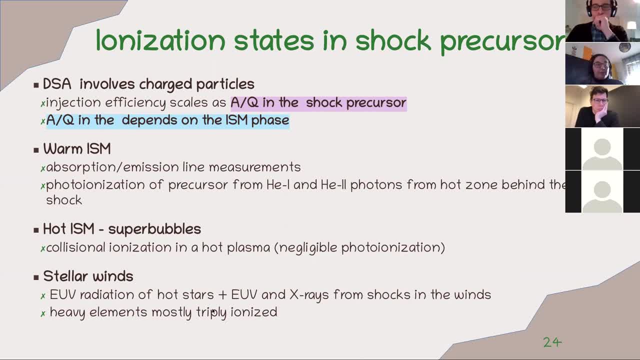 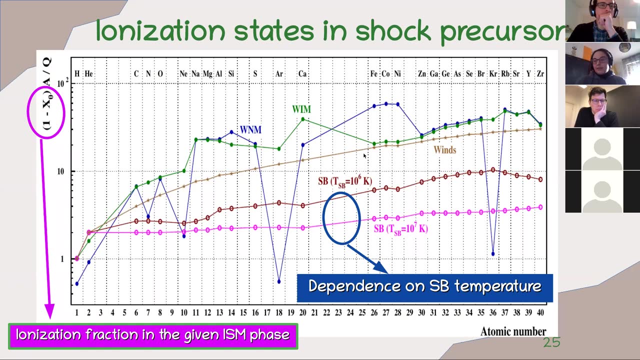 And there are models that show that in this environment, most of heavy elements are basically triply ionized. So So, So, So, So, So So. helium would be fully ionized, the others triply ionized. And from all this information and models we extracted, 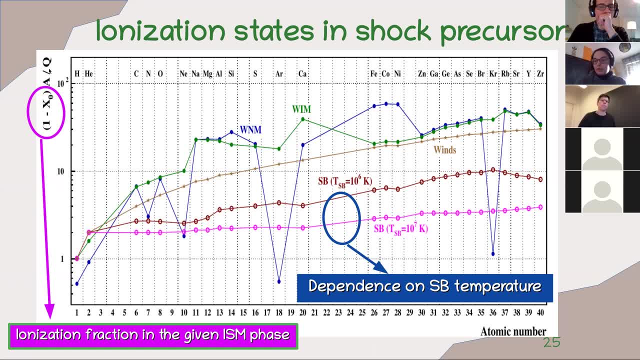 an effective mass overcharge ratio corrected by the ionization fraction found in a given species and in a given ISM phase. And we see that the dependence on the ISM phase is quite large, because here we have this is the warm, neutral, medium warm. 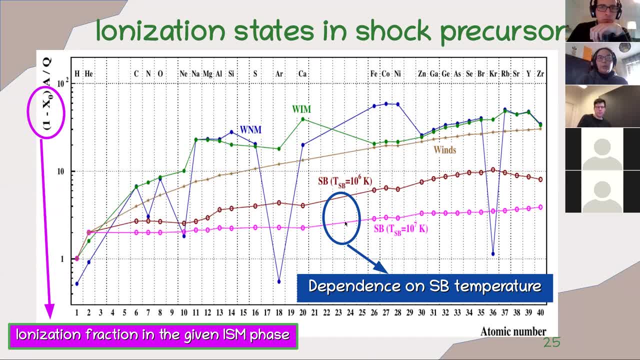 ionized wind And also when we look at super bubbles. there is a strong dependence on the super bubble temperature, And this is important because we allow us to disentangle the origin of cosmic rays in the various gas phases. And so we built our 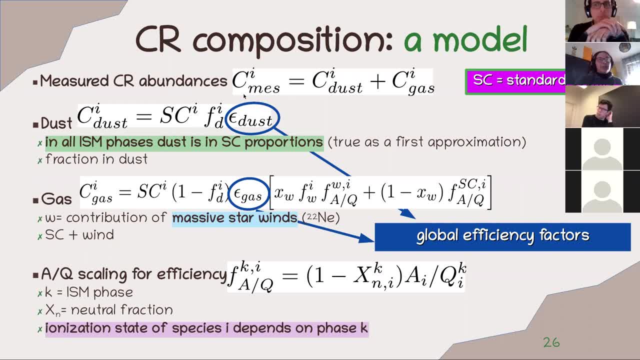 model in which we assume that they measure abundance of a given species E. It's contributed by dust, grains and gas and, depending on the species, could be mostly dust or mostly gas or a mixture of the two. And that because so we start with the standard composition of 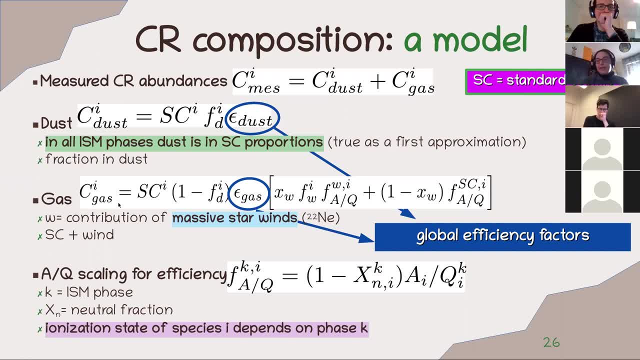 the interstellar medium and for each ISM phase we introduce the some factors that provide the correct abundances, ionization factors for each phase. So I will try to summarize this. So for the dust, for instance, so for each species E, we have that. 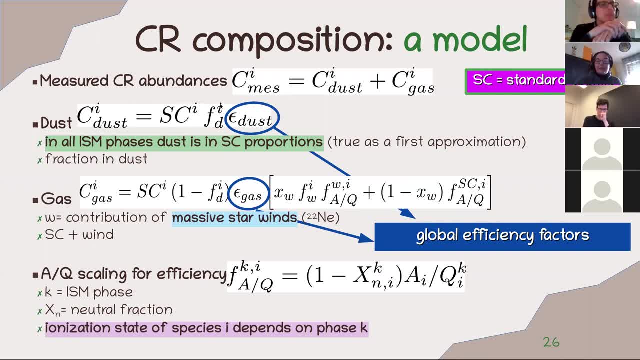 the standard cosmic composition with a given fraction in dust would be accelerated with an overall effusion, So that's what we call the Epsilon dust. Since we do not know much about the distribution of dust grains in the various phases, as a first order approximation we assume that 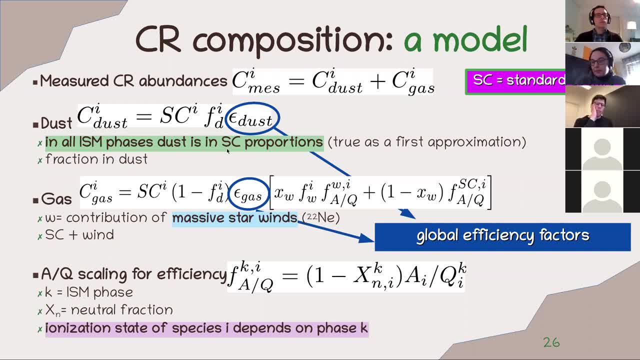 in all phases. dust grains are the standard cosmic proportions. Unfortunately, with the information that we have, it was not possible to do better than that. Then we look at the gas phase contribution. So we have the standard cosmic composition, With the fraction in gas an overall efficiency. 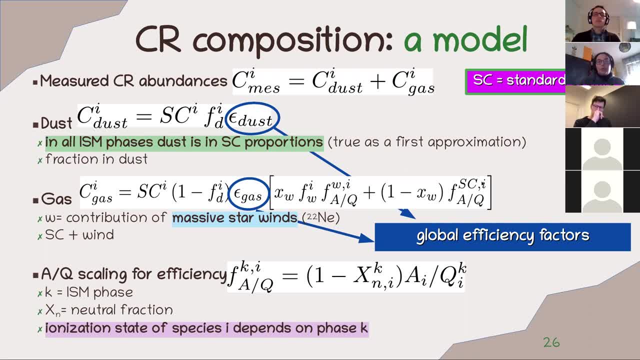 And then we have the contribution to acceleration of gas, which depends on the A over Q ratio. As we have seen, the efficiency will scale as A over Q, And so for each species we have the effective mass over charge ratio, And we have the wind contribution that will provide the Neon 22.. 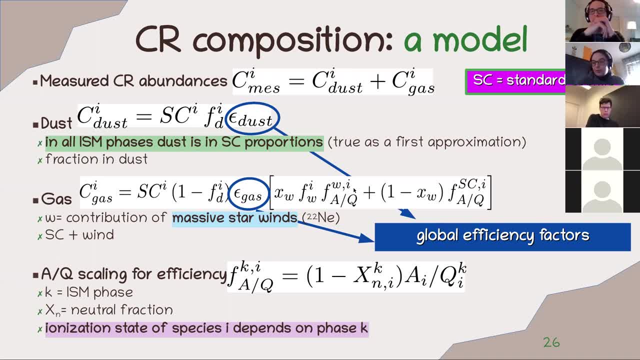 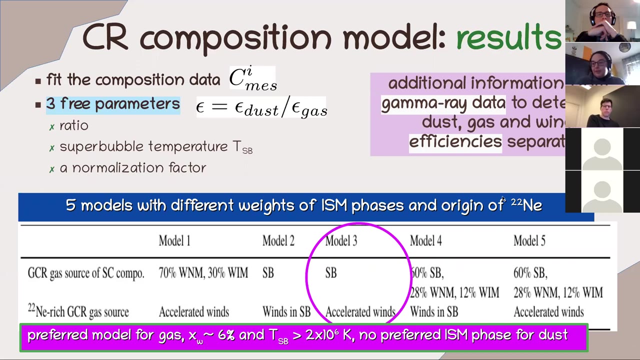 And also, in this case, we have the average A over Q associated to the wind phase, And so this was done for every species and for every ISM phase that we consider. Finally, we put together all these things And we create five different models in which we assume that the contribution from different ISM phases 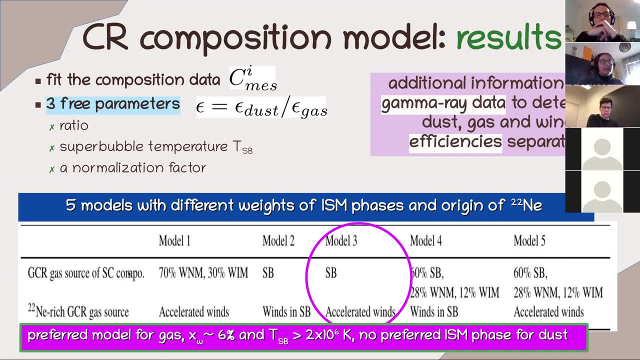 to the gas phase is different. So we have a model in which most cosmic rays are accelerated from warm phases only, or from super bubble only, or from a mixture of warm phases- only the two. And also for the wind material we assume different. 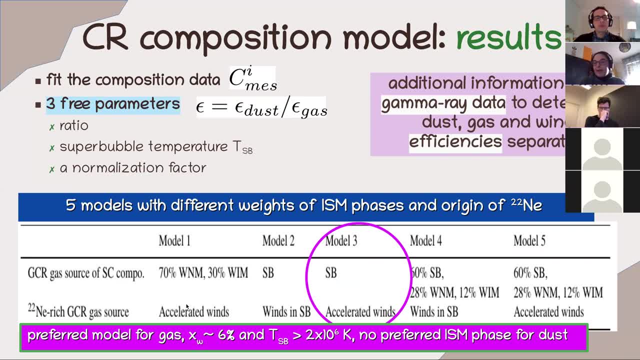 scenarios in which either the wind is direct, so the wind material is accelerated by supernova remnants, or winds accelerate directly the material, So acceleration and the termination shock of the wind, or acceleration of a mixture of interstellar and wind material. So, if you are 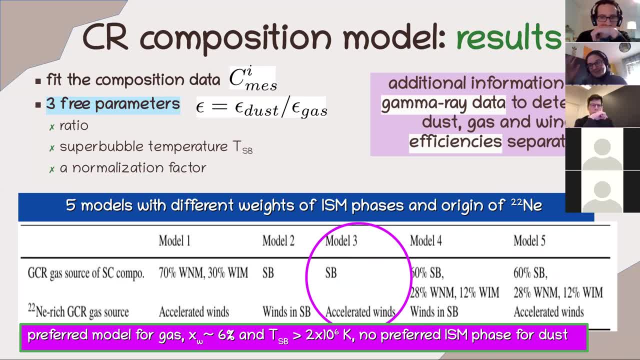 interested, you can look at the details in the paper. So I know that it's a lot of detailed information. I'm sorry for that. Anyway, in these models there are three parameters which can be extracted. So these three parameters are the ratio between: 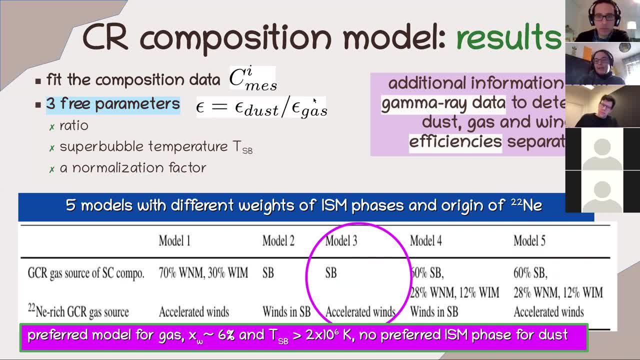 the overall acceleration efficiency of dust and gas, the superbubble temperature and an overall normalization factor, And we can extract these parameters by fitting the measured abundances. Moreover, we have an additional information, as we will see in a while, from gamma-ray data that allow us to disentangle between: 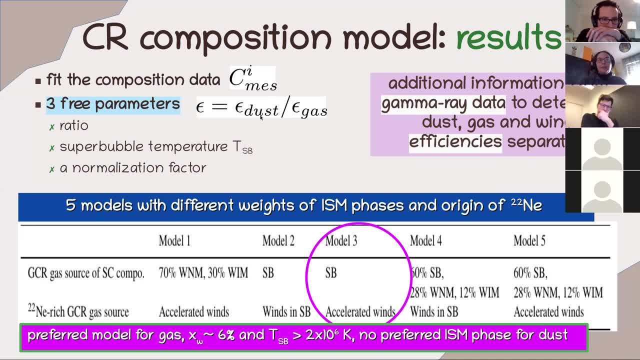 the overall acceleration efficiency of dust and gas. Anyway, from our analysis we saw that the preferred model is this model tree, in which the main galactic cosmic ray source is a superbubble environment and with a direct acceleration of wind material at the wind termination shock for providing the NEON22. 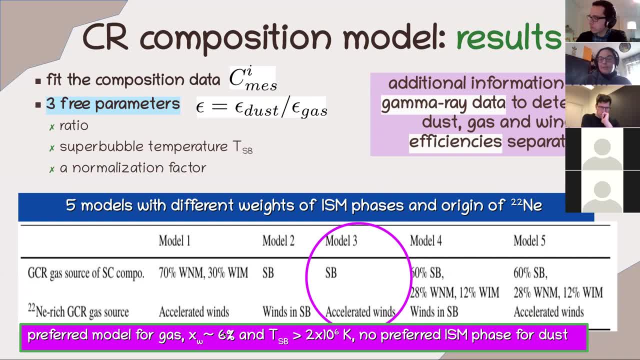 And the wind material should contribute for the 6% and the superbubble temperature should be somehow larger than something to 10 to the 6 Kelvin. And, as I said, there is no preferred phase for dust because we do not have information on how dust is distributed in the different phases. 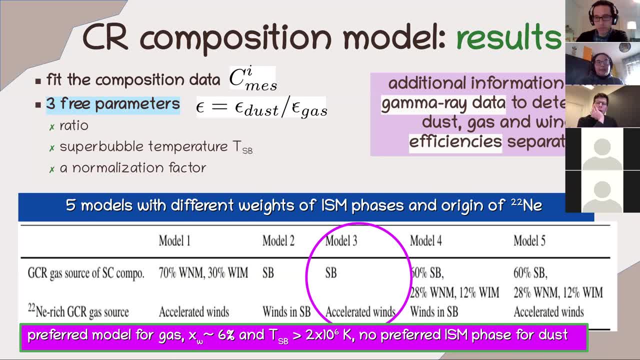 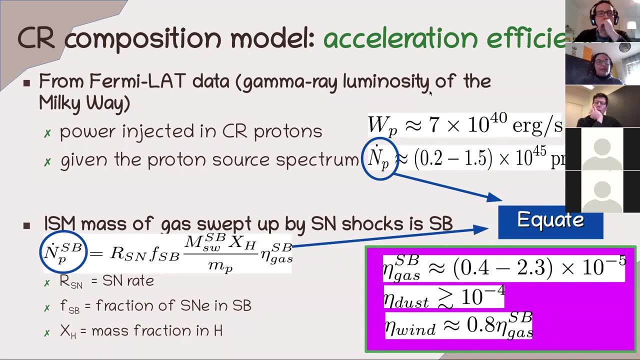 But from this model, as I said, we can extract the ratio of acceleration efficiencies of dust and gas, but we want an information of the two separately. And how can we do that? We by using gamma rays. Indeed, as I said at the beginning, we know from gamma rays. 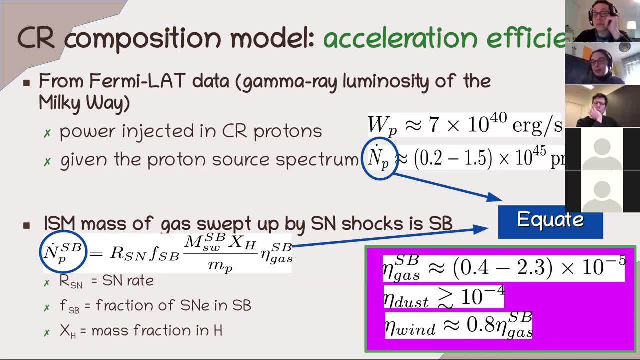 that the cosmic rate distribution in the galaxy is more or less uniform And we have an overall power associated to that. And this power is also associated to protons which produce these gamma rays. So once we know from our model the source spectrum of protons, from this information we can extract on how 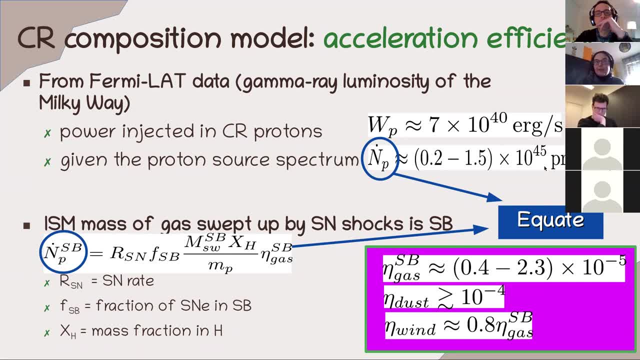 many protons are injected by sources per second And we get this number. So this is an independent information. just looking at gamma rays, On the other end we said that superbubbles should accelerate mostly cosmic rays. So we can compare the number of protons. 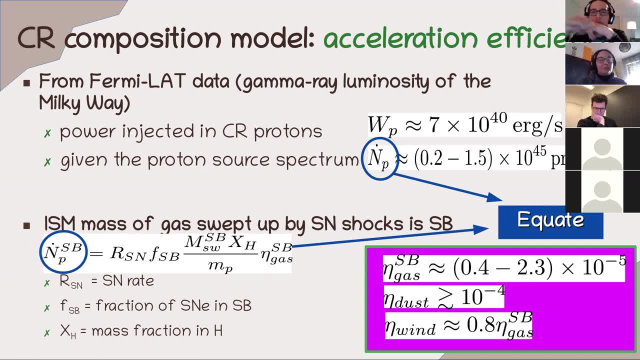 injected by supernova remnants that accelerate within super bubbles per second to this number. Thank you, How do we get this number of protons per second? Basically, we have that each supernova that explodes in a super bubble during its lifetime sweeps up a mass given by this number. 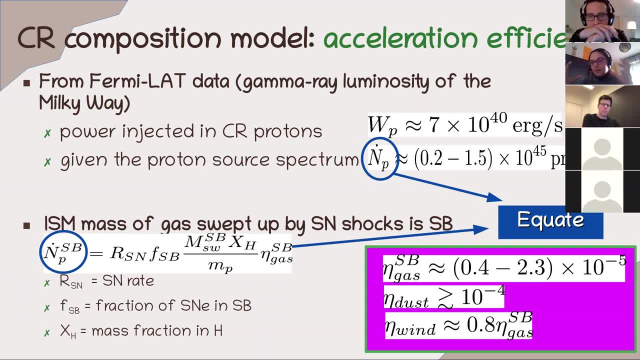 And this can be computed easily, because we know how a supernova expands in a given medium And then we have the fraction of mass that is in hydrogen And from this we know how many hydrogen particles are processed. Then we know the rate of explosion of supernovae in the galaxy and the fraction of it that it explodes within super bubbles. 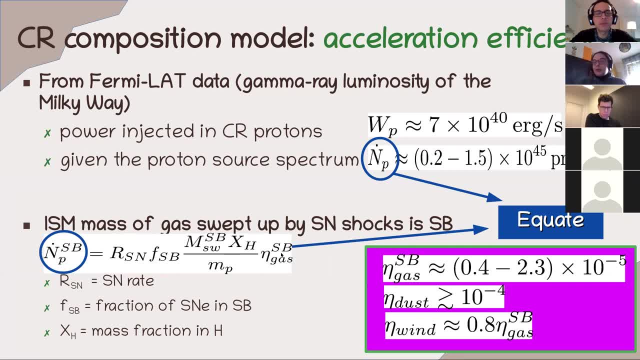 And the acceleration efficiency overall will be a number that we want to calculate. So by equating these two numbers we get our overall efficiency for acceleration, The acceleration of gas for protons, which is 10 to minus 5.. Then for all the other elements, there will be the scaling with the mass overcharge ratio. 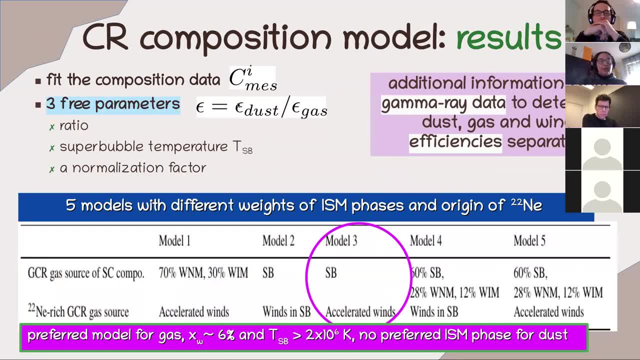 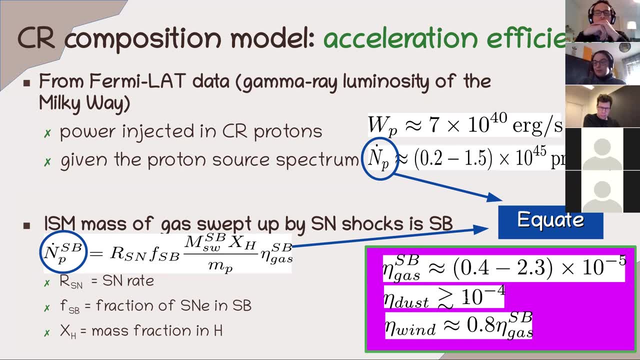 But then fitting our model. previously we knew the ratio between dust and gas efficiency, And so from that we can extrapolate also the efficiency for dust, And the same we can do with the wind material. The acceleration in the wind is similar as efficiency to that of gas. 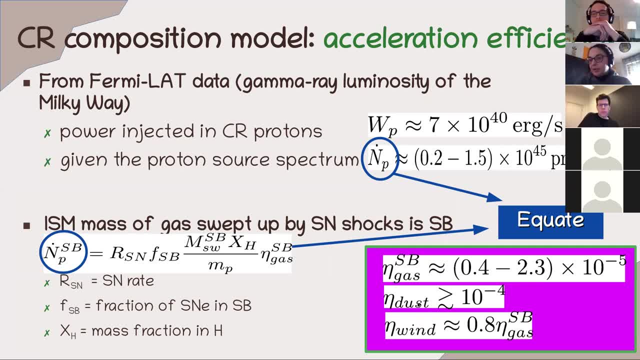 But the acceleration of dust is much more efficient, as we have seen, due to dust grains acceleration. The interesting thing is that in the seminal paper of 1997 of Meyer and Ellison that provided the first estimate of the acceleration efficiency of dust grains, They got a similar number. 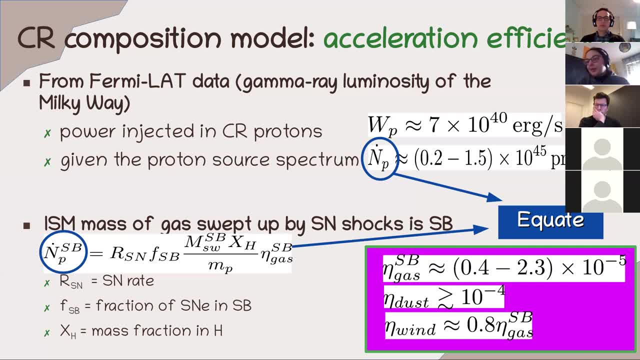 So somehow our work is consistent with the only other information that we have from acceleration efficiency. So far, this number is not being confirmed by simulations, in the sense that the only simulations that provide the number of acceleration efficiency It's the one of Caprioli et al 2015.. 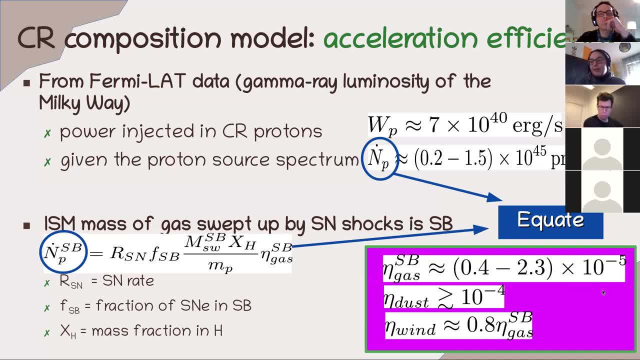 So we get a much larger efficiency of the order of 0.1 or 0.01.. And we do not know why there is this discrepancy, And so let's hope that in future works we could understand this better. But from our analysis, this is the number that we get. 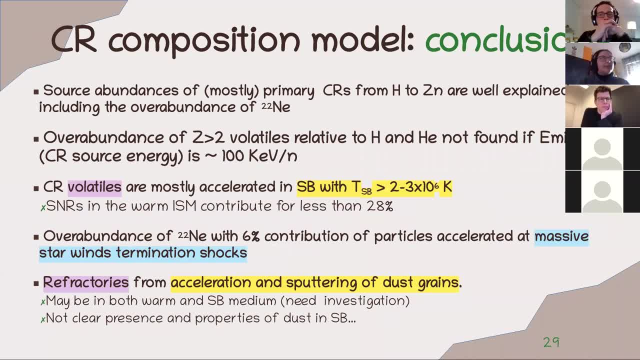 So I will briefly go to the conclusions of this talk. So what we did was to investigate The abundances of cosmic rays at the sources. So namely we consider mostly primary cosmic rays, from hydrogen to much larger nuclear, And we were able to explain the composition. 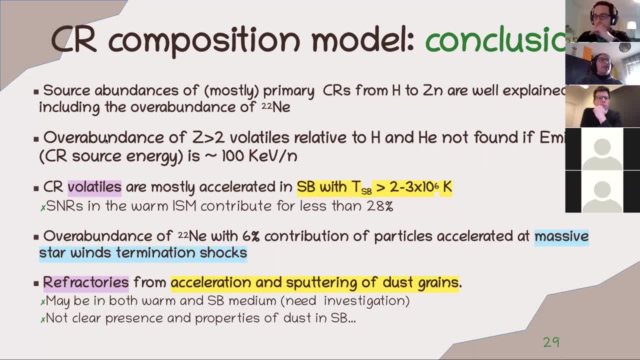 Also including the overabundance of Neon 22.. From our analysis we were able to show that The minimum energy from which we Integrate the source spectrum of hydrogen and helium It's 100 kV per nucleon. There is no overabundance as it was previously suggested. 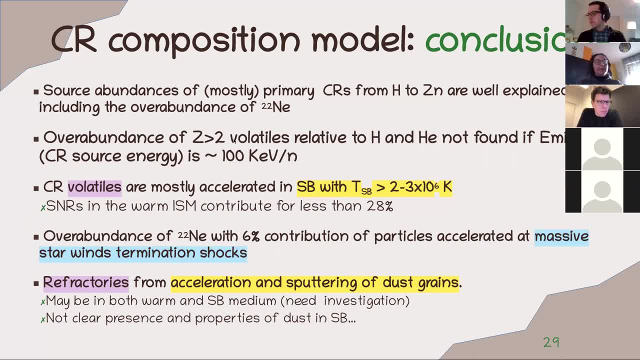 But this needs to be further investigated. We confirm that cosmic ray volatiles are accelerated less efficiently than dust grains And that such volatiles are likely accelerated from super bubble environment, And we also estimated the maximum contribution from other phases, So namely from the worm ISM. 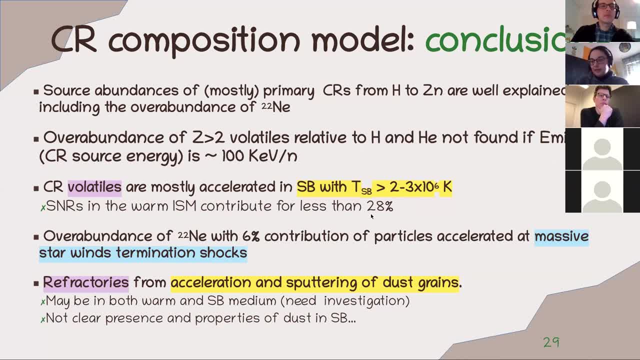 And from our analysis it seems that this contribution should be less than 28%, And the overabundance of Neon can be explained with a 66% contribution Of accretion Of wind material At the wind termination shock of massive starts. 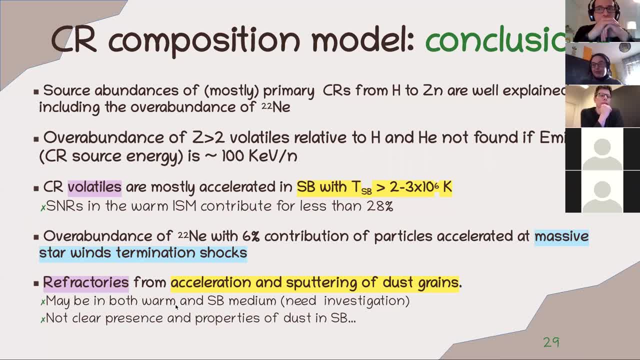 And the refractories, as previously suggested, are accelerated very efficiently And the material that is accelerated, then it's spattered, Thus injecting the refractory elements with large efficiency. But unfortunately the present data that we have done Does not clarify. 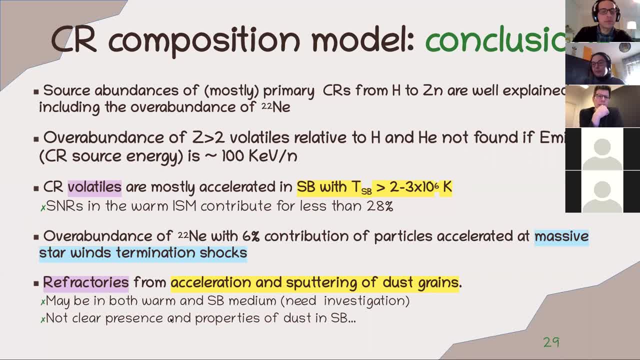 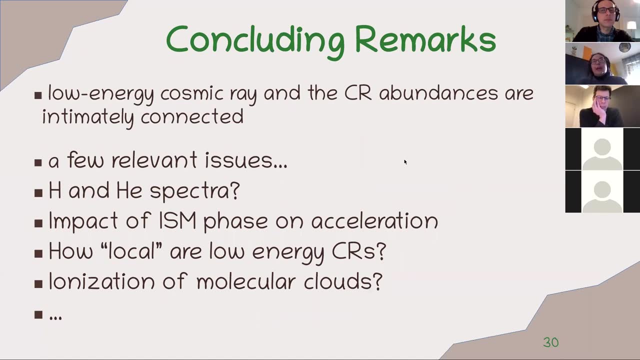 Which is the composition of dust, grains And presence in super bubbles And in other ISM phases. So this should be clarified in the future. A few concluding remarks. So when starting to work on this topic, I realized that the cosmic ray composition probably is one of the less understood things in cosmic ray physics. 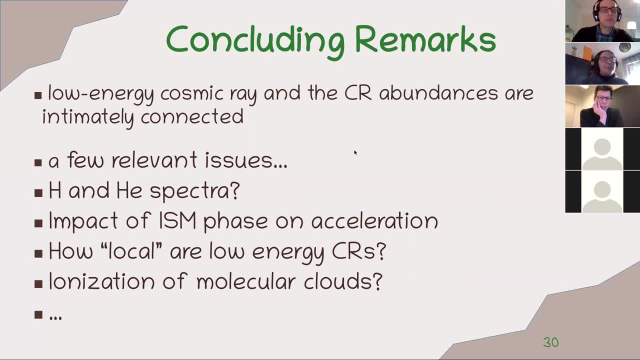 And there is not much work on it, Probably because it is somehow unpleasant to work with it Because you have so many details And also from the point of view of observations. So you need to go to low energies Where things are not well understood. 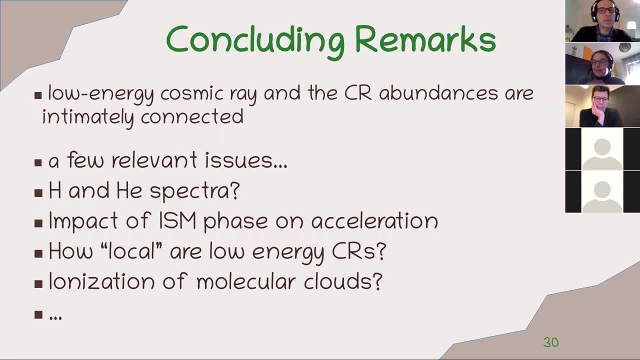 The data are probably less present at higher energies, And many other issues remains Which are connected to the fact that we are looking at low energies. So, for instance, this discrepancy of helium and hydrogen spectrum, Which to me is quite puzzling And, in my opinion, should be addressed in the future. 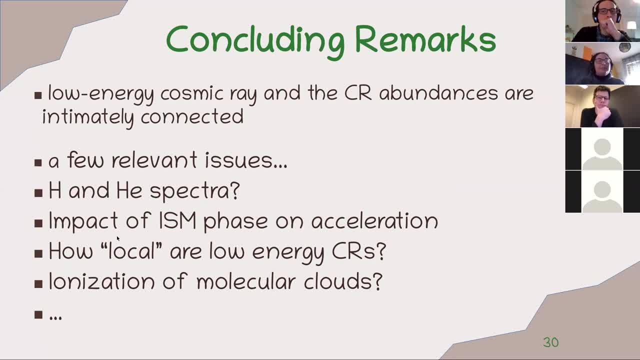 But also there is this problem of, if we look at low energies, We are sampling, probably something which is local, Due to energy losses, And so also in my opinion, It would be important to understand whether the data that we are relying upon To understand the composition. 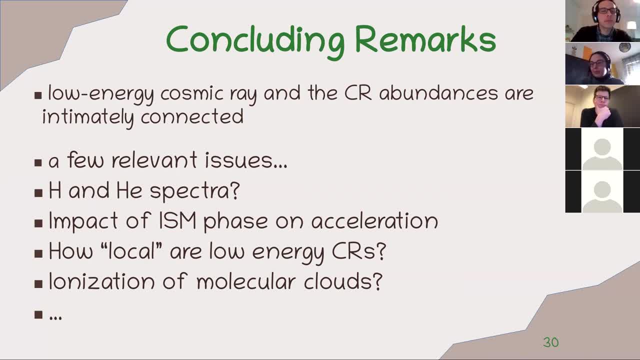 Are really average cosmic ray population, Or what is the role of local sources. So this is something that probably in the future we will try to address, And so this was my talk And thank you for your attention. Thank you very much, Sarah. 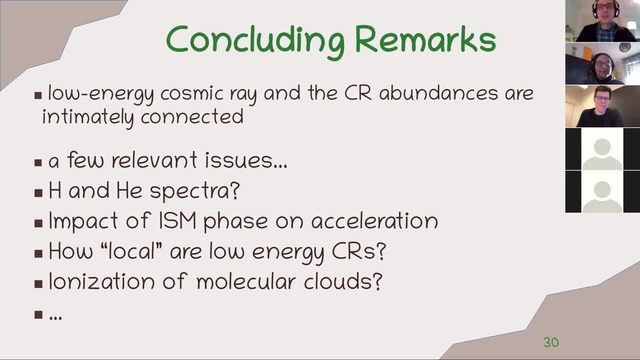 This was very comprehensive. There's lots of stuff to discuss. I'm sure We have maybe time for two or three quick questions, So just yeah, I think Markus has one. Thank you, Sarah, for this talk, Can you? So? you mentioned that you. 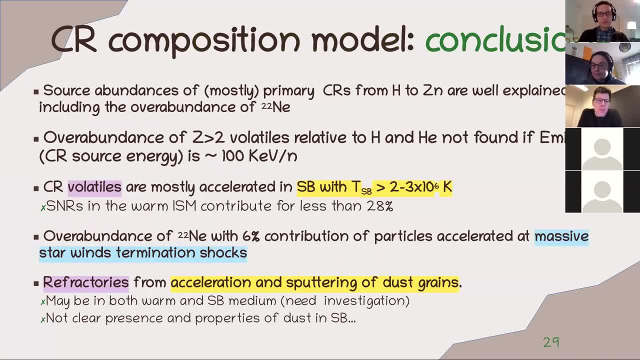 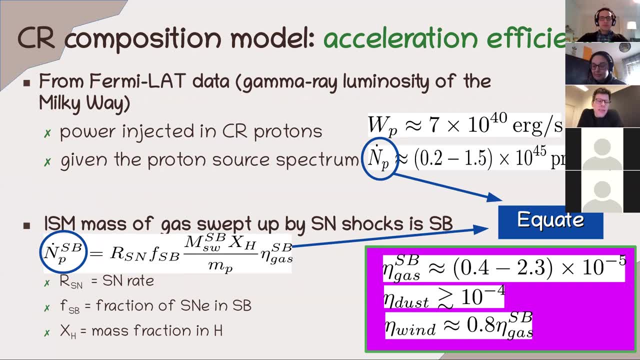 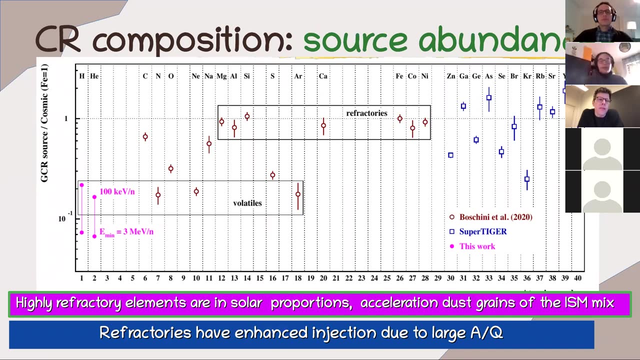 So you fit cosmic ray data with your three parameter model. Can you say again What exactly you mean with cosmic ray data? Is this just the Relative composition? Yeah, The composition data, This one, Yeah, Okay, Yeah, So it is this kind of data. 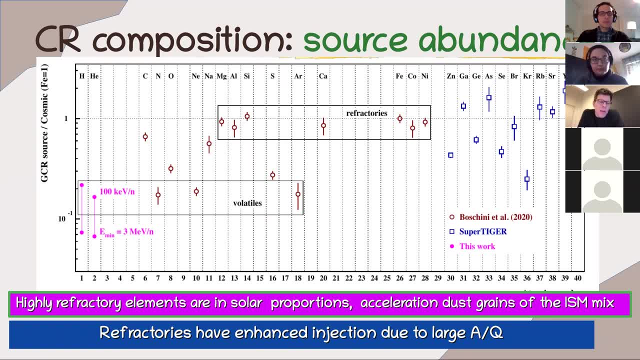 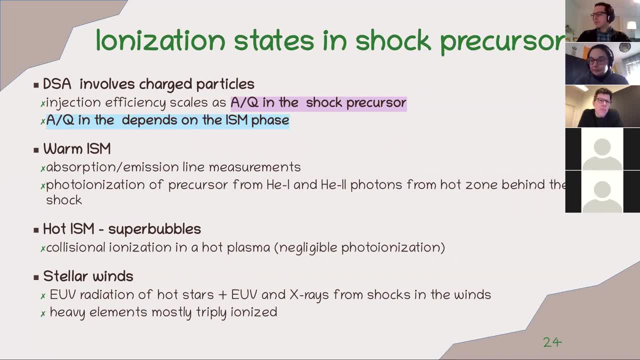 And then, for example. So one of the parameters was the, The temperature of the super bubble environment. So is this going to influence the Dynamics? This is going to Give you the Fraction of ionized material that you inject into your shock, or 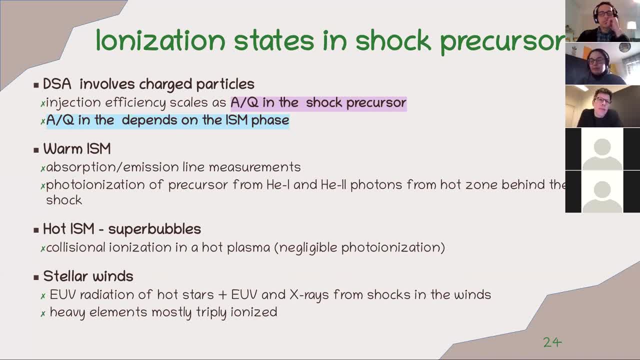 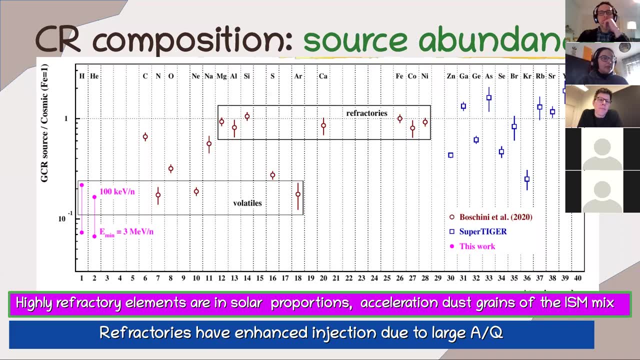 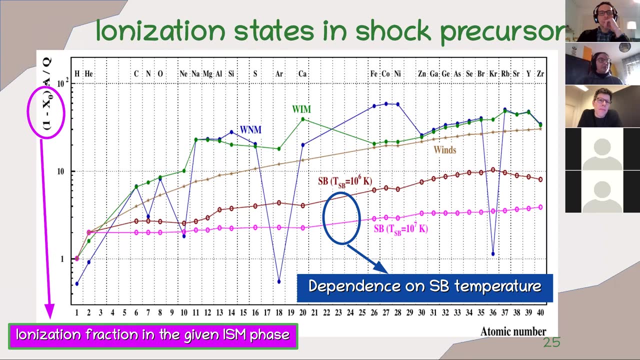 Yeah, How does this Now? this is So, for what matters is important for the ionization state in the shock Precursor. So there was this, Maybe Yes, So you see that If you go and look at the average mass over charge ratio, 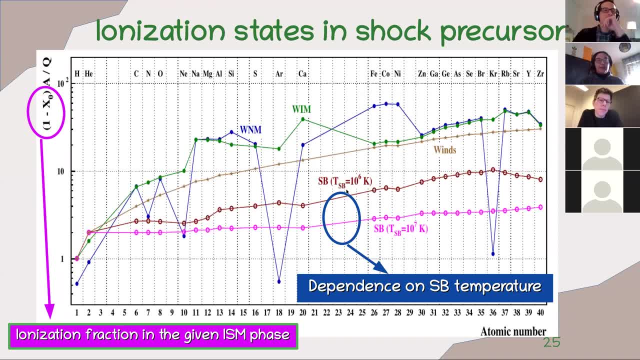 So if we look at 10 to the six Or 10 to the seven, There is a difference, And so this will affect The way in which cosmic rays are injected and accelerated. I see, Yeah. Thank you, Enrico. 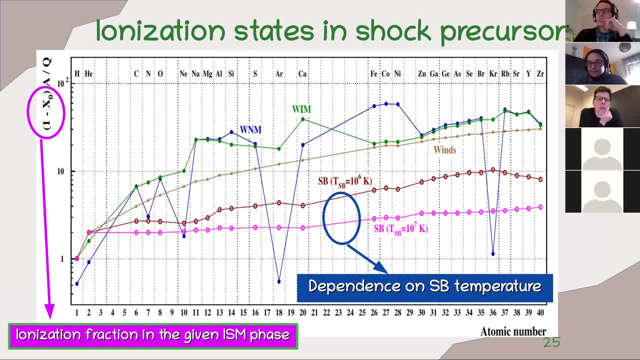 Yeah, Thanks. First of all, Sarah. It was very nice, And I have a Couple of questions. The first one is a Curiosity: So you said That at the end you're able To work with the? 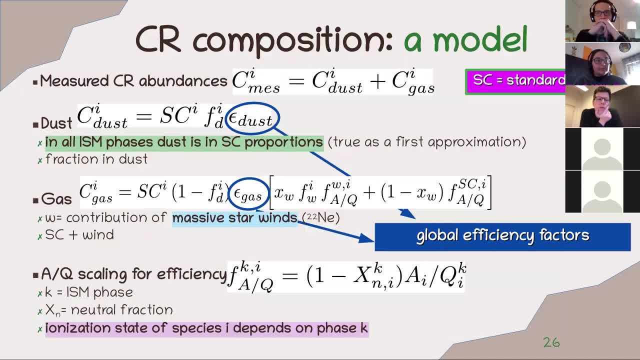 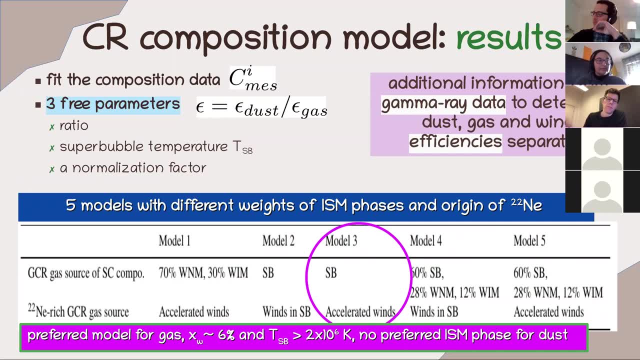 With the Three free parameters, And I was. I was wondering Which is the level Of degeneracy that you get in your conclusions, So Especially on this Epsilon, which is the ratio, And With the other two. 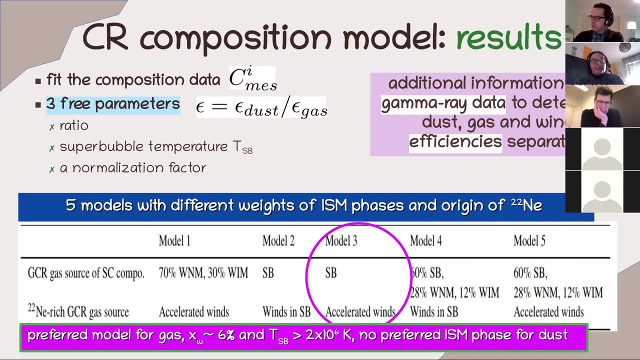 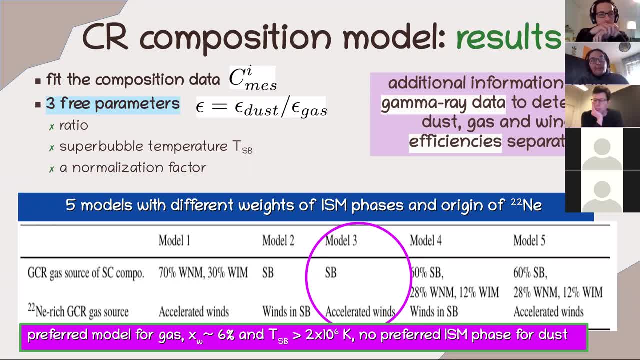 Or Which Are the observation That allow you to To break, Because maybe I lost this part. No, Okay, Yeah, So From this model, So From the Composition, We only Can get An information. 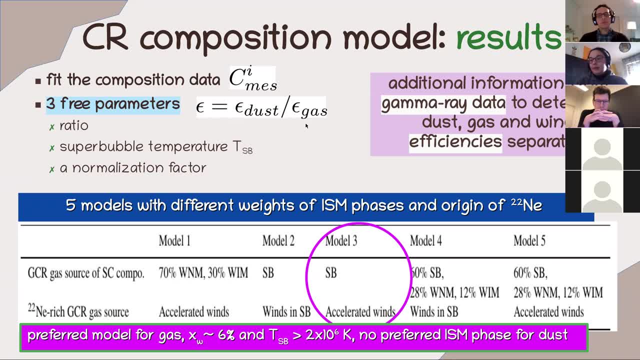 On this, On this ratio And The level Of degeneracy Depends On this That You Consider, And In the analysis Is Post Shown That There are. This model Provide. 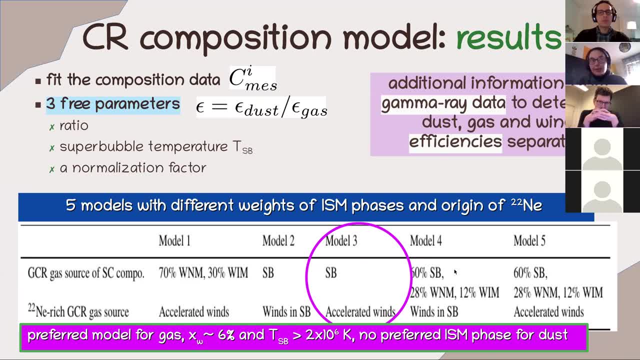 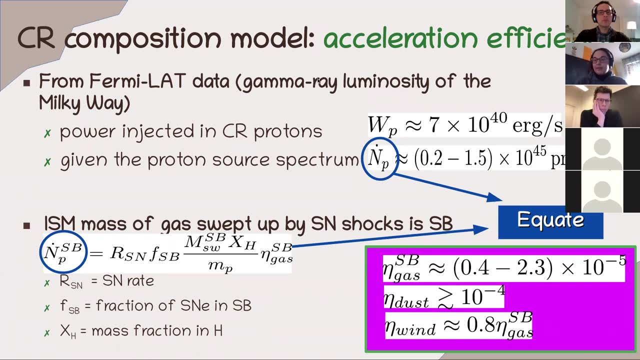 The chi Square, Which Is Evidently Smaller Than The other These Other Models. So I Didn't Show That, But It Is Because, Basically, Using My 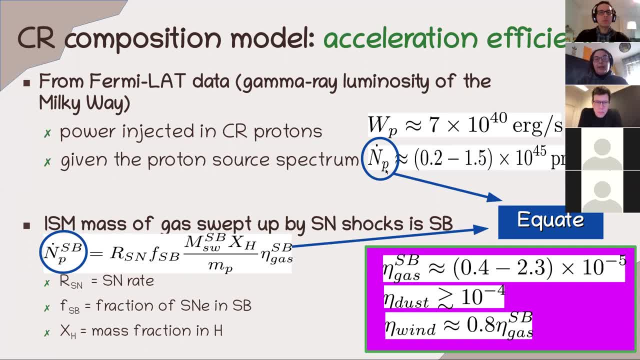 Information On Protons. We Were Able To Extract, At Least For Protons, The Acceleration Efficiency. So Once You Know That Particles Are Mostly Accelerated, 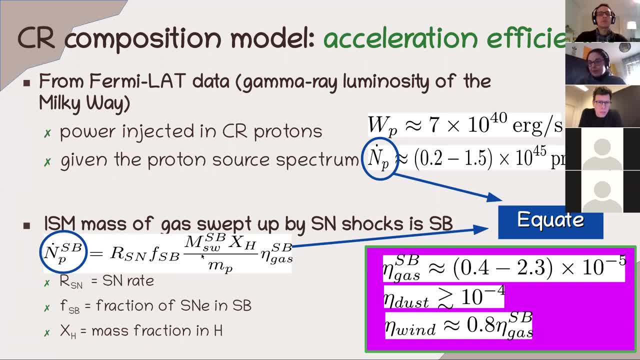 I Know You Know How Many Matter Is Processed, So How Many Protons You Put In Front On Efficiency, And Then You Know The Outcome. 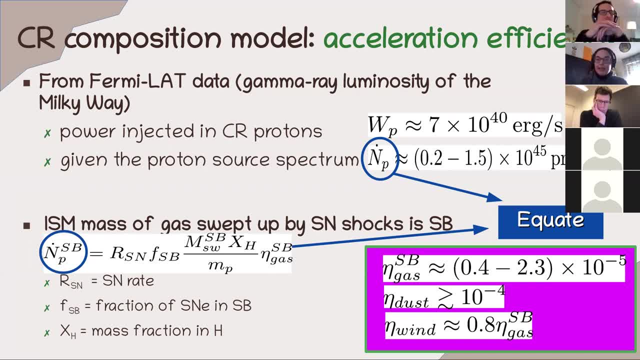 Because The Same Protons. You Just Rescale It With The Mass Overcharge Ratio. Is It More Clear Now? Yeah, Yeah. So This Leads Me. 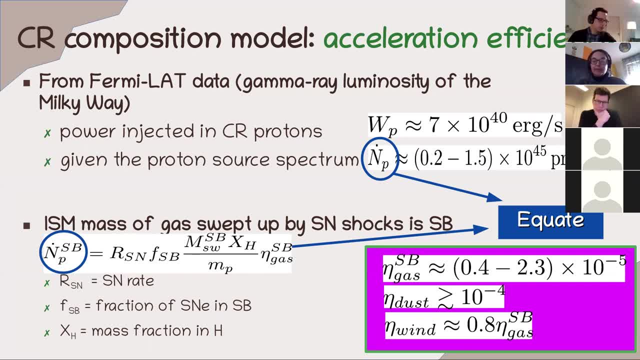 To The Follow-up Question, Which Is So If I Could Be So Sort Of Problem For The Standard Supernova Remnant Paradigm In The Sense. 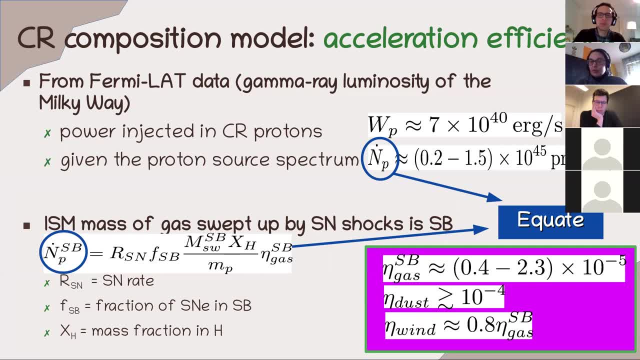 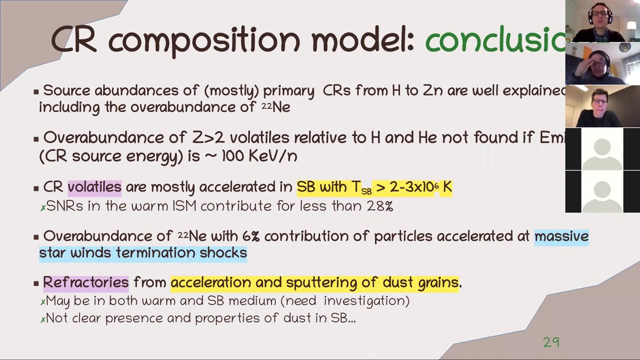 That We Are Having Being Supernova Exploding In The Super Bubble, But At The End Of The Cosmic Race. No, We Have An Additional Information. 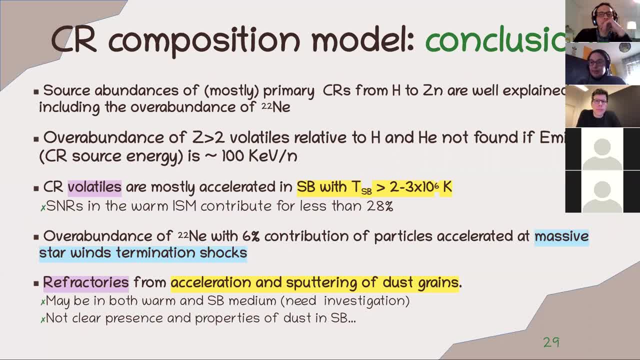 On That Because, Okay, So Supernova Will Remain The Main Source Of Super, Of Cosmic Race And They, If Most Of Supernova, Explode Within. 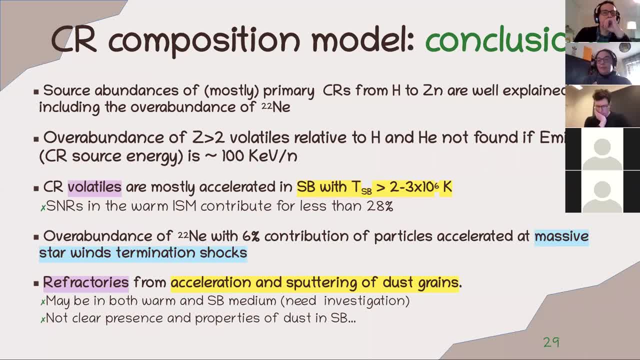 Super Bubbles, So Maybe It's Not So Crazy. The Information About The Wind Termination Shock Contribution Is In The Neon 22. And So We.